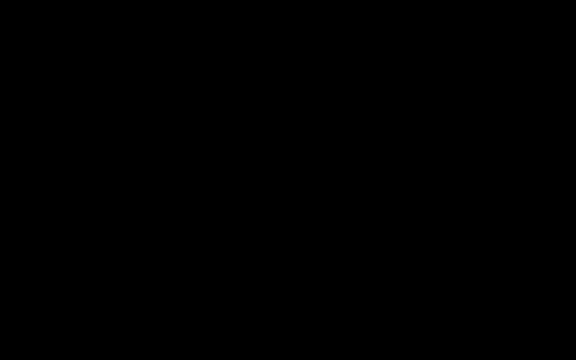 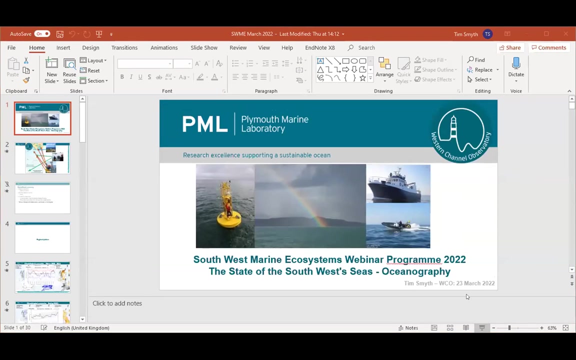 sharing my slides, so just bear with me And you should hopefully be able to see that in presentation mode. Is that all good to people? remote Keith, can you see the screen there that I'm sharing? Yes, I can see the screen. You just need to open the PowerPoint. 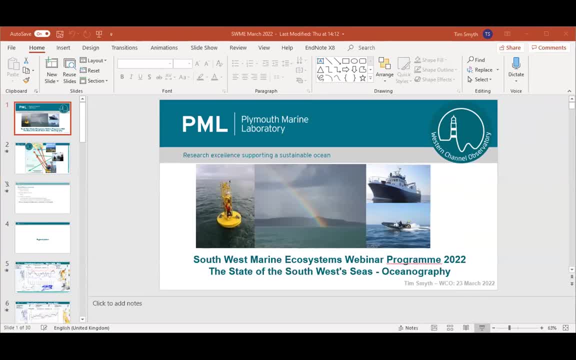 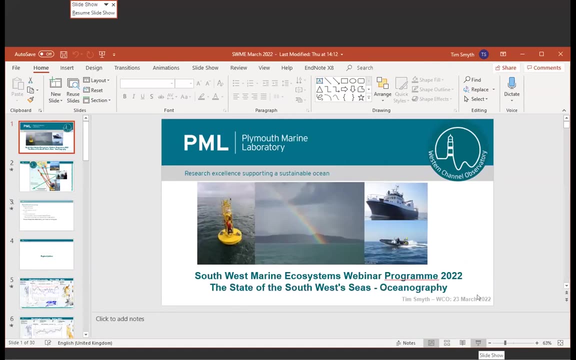 I'll have opened the PowerPoint and I'm hopefully sharing in presentation mode. No, it's not in presentation mode On your computer screen. That's what I've got. Yeah, I'm the same. It's not in presentation mode yet, Tim. 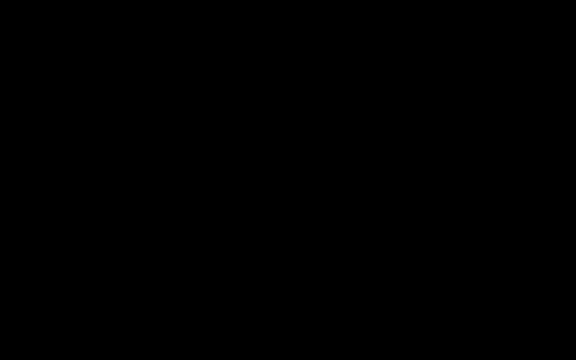 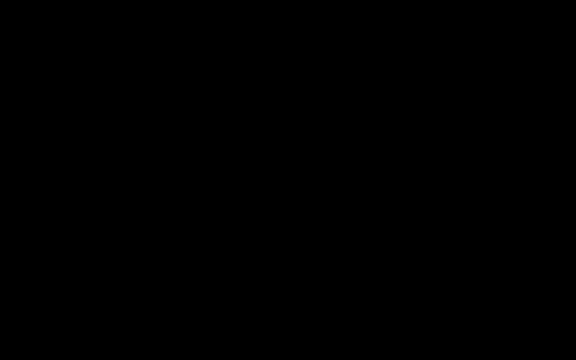 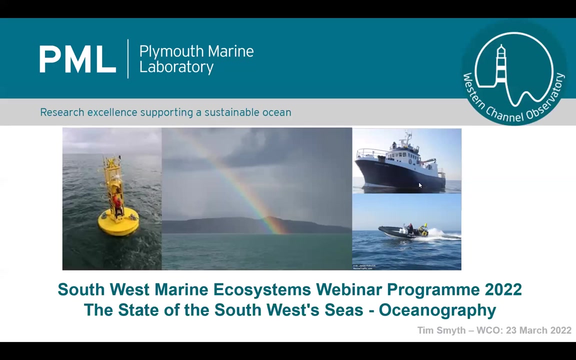 Okay, Okay, All right, All right, Great, All right. Hopefully now you can see it. Indeed, we can see that. Thank you very much indeed, And thank you very much to the MBA for hosting this seminar for us. So what I'd like to talk about today is the state of the Southwest seas. 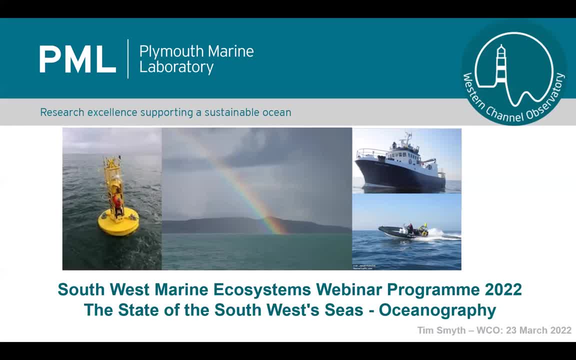 we've called it oceanography, but actually it's more probably the salient meteorology which then drives the oceanography, and the talk really will be centered around the observations of the western channel observatory over the past 12 to- let's call it- 15- months, because i'd quite like to capture 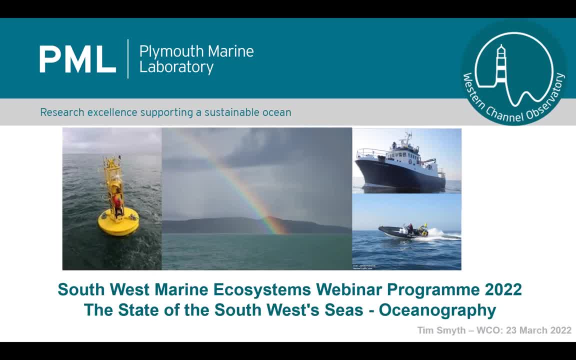 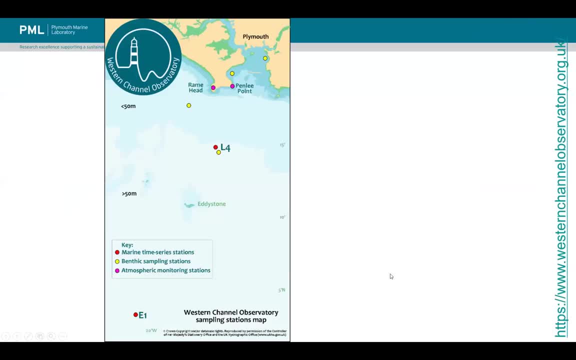 some of the latest events that we've been seeing since the start of the new year. so hopefully, advance the slide. so what is the western channel observatory? so, to those of you who don't know what the western channel observatory is, it's really a a set of time series, stations. 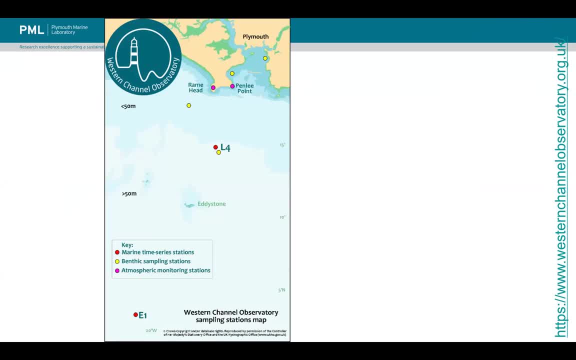 in the western england channel um and the major marine time series stations are highlighted in red. so that's station l4, which is about uh four nautical miles due south of of rame head, and then station e1, and then station e1 and then station e1. 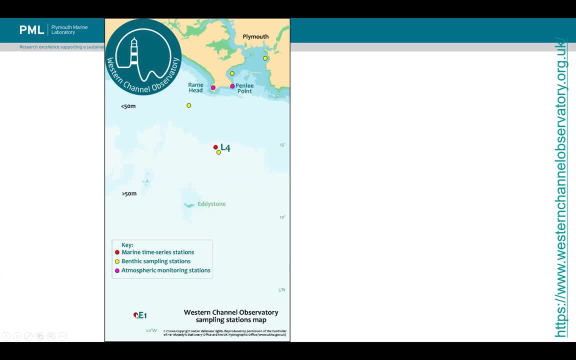 which uh go, which is about 20 nautical miles uh off uh rain head. and then, if you think about how far the eddiston is away from plymouth, uh, pretty much the eddiston reef bisects um l4 and e1 l4. 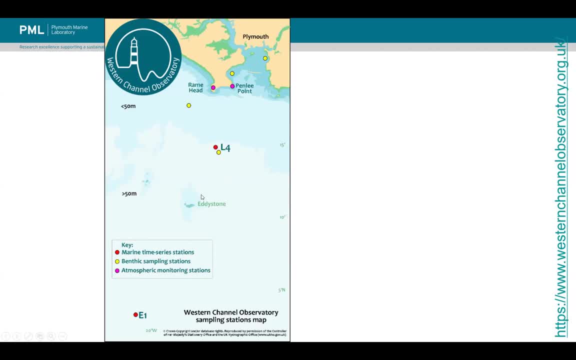 is in around about uh 50 meters deep uh water and station e1 in about 80 meters deep water. l4 is much more coastal in its nature and e1 is much more sort of open shelf uh in its hydrography. um we've also got several other uh parts of the western channel observatory so we've 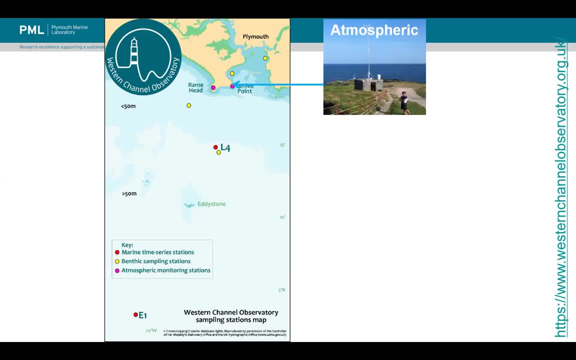 got an atmospheric uh time series station. we started about 2014. uh, really, looking at the atmospheric chemistry of what's going on. so that's the old trinity house, or the trinity house hut, um, which if you walk around the coast you'll, you'll know it very well, uh, and we've been. 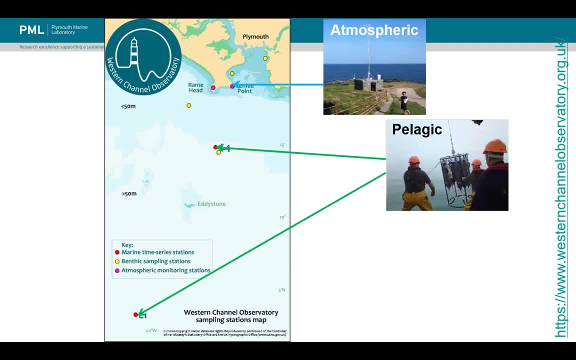 taking measurements there for about the last seven or eight years um the pelagic time series i've already mentioned, so we take uh water samples uh and ctd with depth at uh the the two uh marine time series stations. there's a an image on a very calm day of the uh ctd rosette going over the. 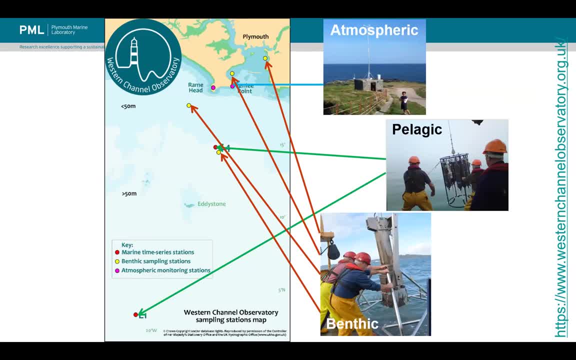 um aft end of the of the quest. and then we've got some uh benthic uh time series stations again at l4, one uh just off rain head and then one at course hand and one at jennycliffe. so these really what uh comprise the, the major parts of the time series of the western. 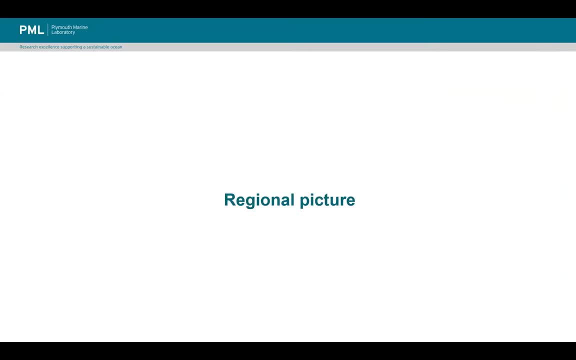 channel observatory. so let's dive straight in as to what the regional picture is going to be. i've taken a lot of this data on all of this data from the uk met office. uk met office, every season, produced this really great um sort of synthesis in pictures of what's uh, what our weather. 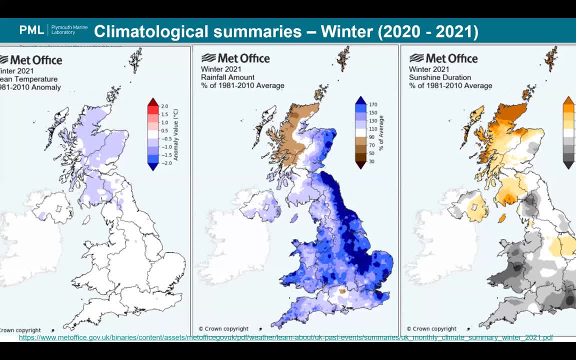 has been like, and i think it's very useful to look at these images. so just to give you a bit of orientation, here on the left we've got the mean temperature, so so the next five slides are going to be very similar, so we've got the mean temperature here. 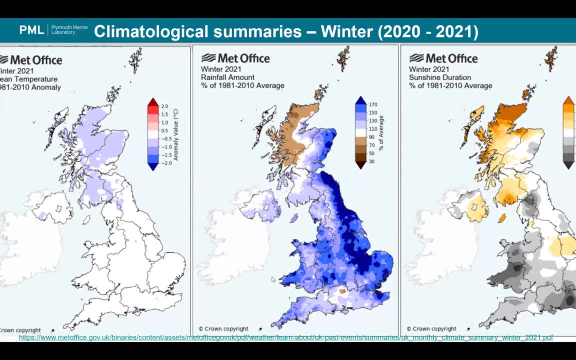 on the left, the mean or the, the rainfall amount in, uh, in the middle, and then we've got this sunshine duration. now, the reason i've chosen these parameters is because, for the hydrography of the western english channel, these things are the things which will drive it so, um, you know how? 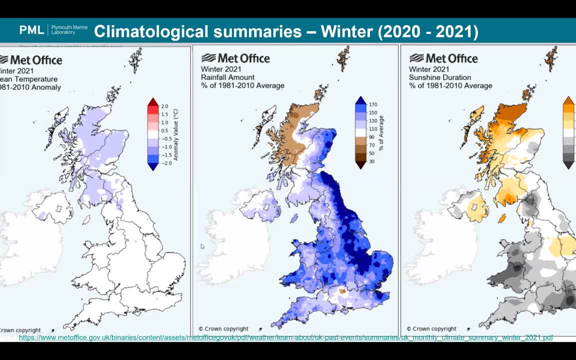 warm it's been, will be driven by the meteorology. the amount of uh, fluvial uh outflow you get from the tamar will be driven by how much rainfall we've had and then sort of the sunshine duration will set the the, the short wave incoming radiation that we get, which will drive things like 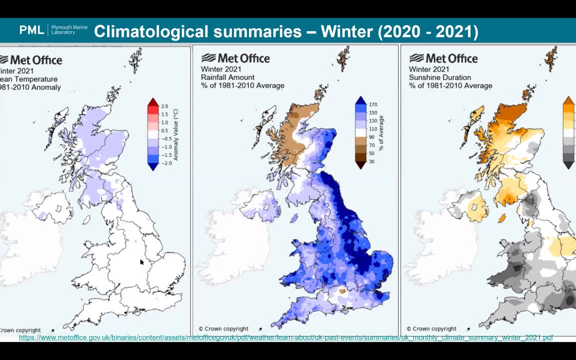 stratification, particularly in the early part of the season. so what we can see here in in the mean temperature, and this is against the 1981 to 2010 um, anomaly um, and what you can see is that pretty much the winter of 2021, so that means the winter from december 2020 through to. 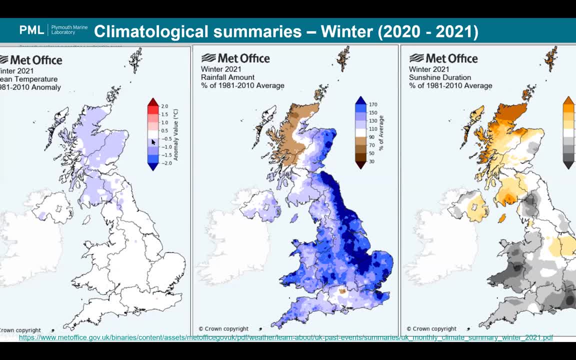 february 2021 was pretty nondescript over much of the uk. um so pretty average um over that period in terms of the amount of rainfall we had. actually it was pretty wet um that, that uh that winter. so the winter before last- um sort of upwards of 110 to 130 percent of the. 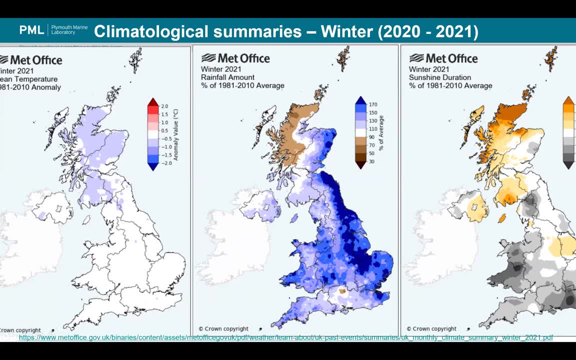 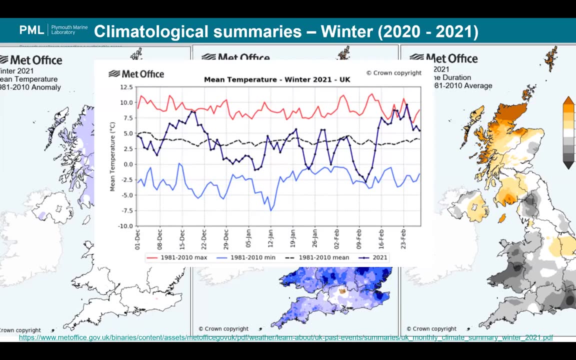 average rainfall that you get and then, as you'd imagine, with the amount of rainfall you get, uh, it was particularly notably uh dull in terms of the amount of sunshine that we got, so that the, the seasonal average uh really sort of glosses over or smears out a lot of the uh of the variability. 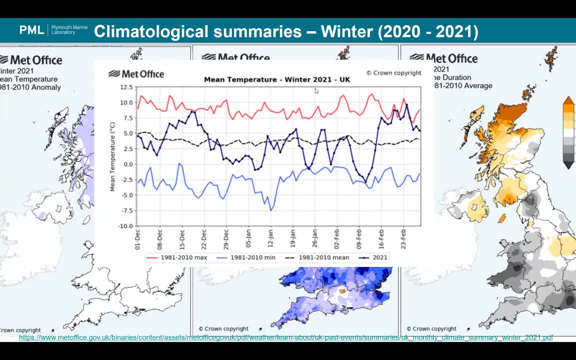 that you get. so what we've got here, this is the mean temperature for winter 2021, with the average shown here in the dashed line, and this, this mean here is the mean for 20- uh sorry, 1981 to 2010, so the 30-year period. now it's important to note here. 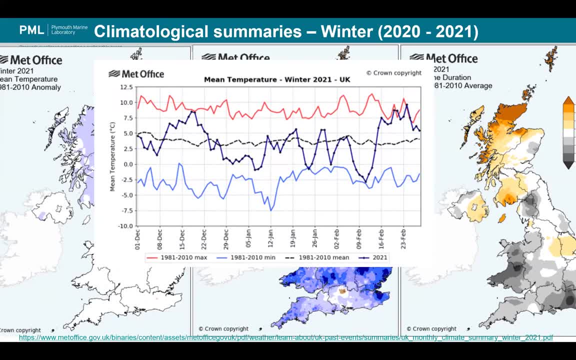 that as we go through into the following uh year, this will change to the 1991 to 2020 anomaly, but this at the moment is uh for that period. now you can actually see here this: this highlights the this, this in uh, this interesting uh period here that you've actually got values greater than uh. 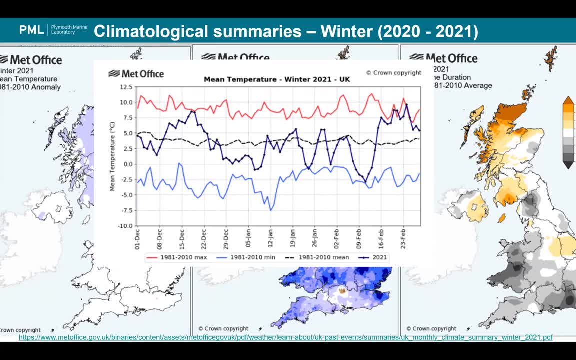 for, uh, the 20 1981 to 2010, max in around february. so what we had here um was a period that was warmer than than in the envelope for 1981 to 2010.. and what you can see is that there were periods. 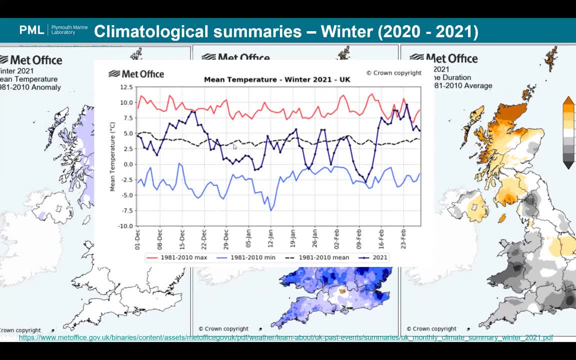 of of colder weather, so sort of the later part of december and into january last year was was was notably colder, and then this period here that we see in uh sort of mid-february, we, we, we went from pretty much the coldest that had been observed in the period all the way up to uh. 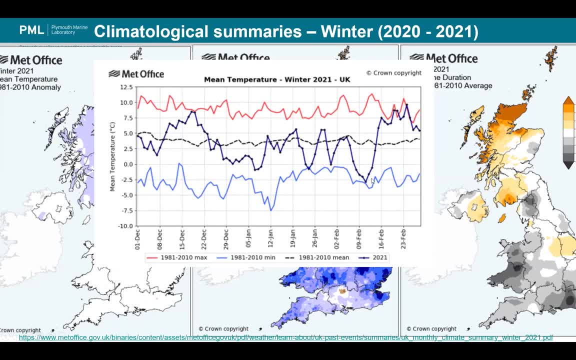 sort of almost the warmest. so, over a period of about a week, there was a notable uh change in the weather uh, which then set the the scene for the rest of the of the winter here. so, although it was a very average winter, there was a lot of variability in it, um, in terms of the temperature. 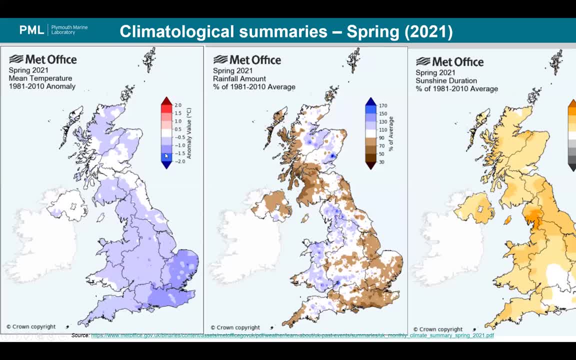 and then let's move on into spring. um, actually, springs, over the last few years um have been very similar to this, that it's been pretty dry but actually quite cold um, and you can see uh that over large swathes of uh the united kingdom that the temperature was almost, you know, approaching uh one degree below uh average. 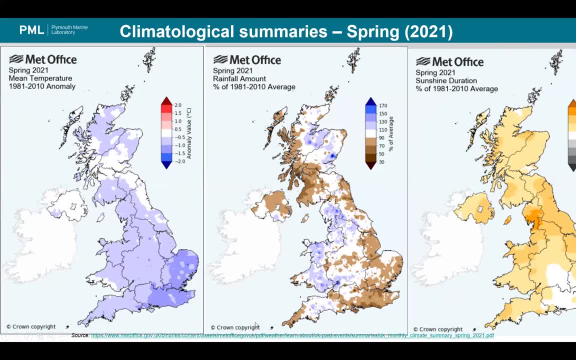 almost uh one and a half degrees in some places of the southeast um. the rainfall itself it was. it was relatively average in our location but if you just go down to the west of cornwood it was pretty dry. so i suppose if we we were going to describe uh spring last year it was cold. 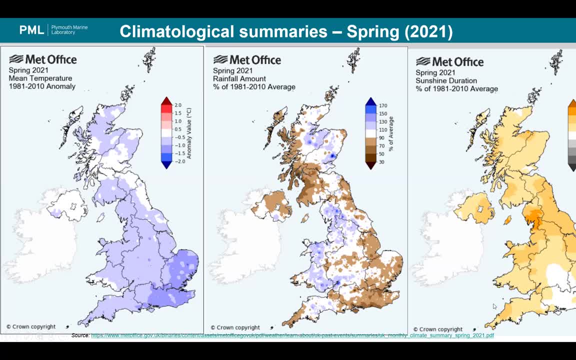 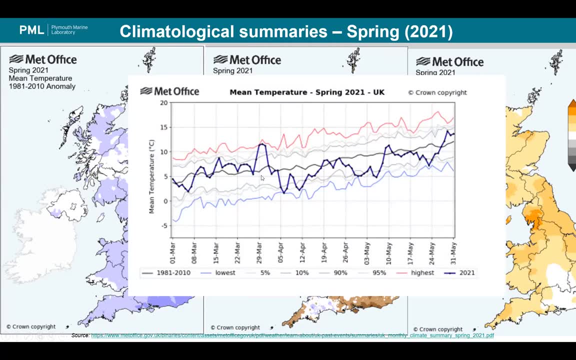 and and and dry-ish, and then we seem to have uh sort of more sunshine uh than the average in terms of what that looked like, in terms of the anomaly. now, what happens here is that, uh, that the met office has kindly added a few extra plots here. so the, the average is uh, the, the, the blue, uh, sorry is. 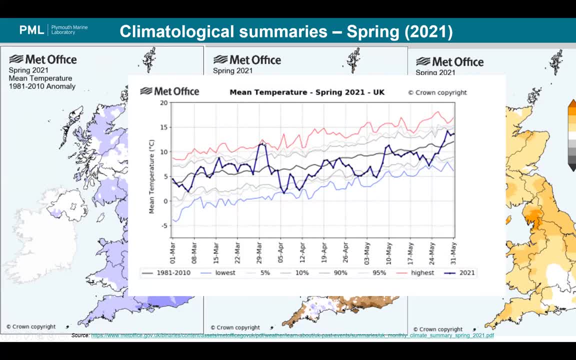 the black line here. what we actually had is in the blue. so you can see that there was a very brief period in in march and early april that was. that was almost as warm as it is as it's got. but then you got this flip-flop right back down to in early april last year, when we had a a notably cold period. 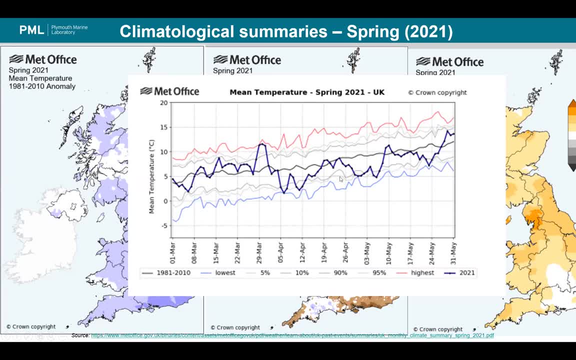 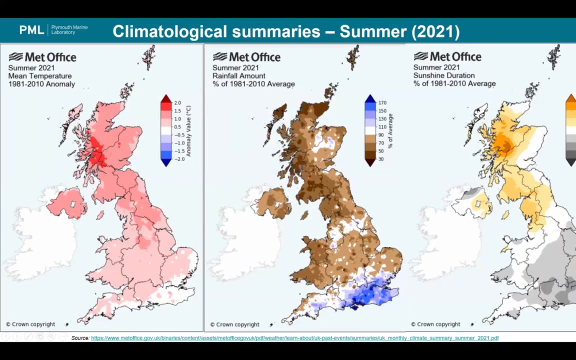 and you can see these. you know there's probably about three notably cold periods in in uh in spring last year and maybe a little bit of a warmth and cheer in this uh sort of latter part of of march. let's go and look at the summer again: summer pretty. 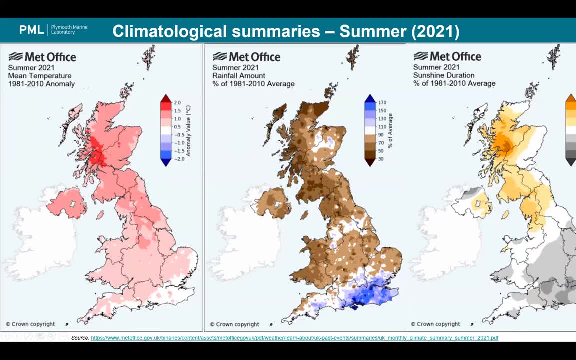 unnotable in our region, uh, so maybe a little bit warmer than average. uh, for, against the 81 to 2010 anomaly, it wasn't particularly wet or it wasn't particularly dry, um, in our region, um, and pretty average in terms of of uh, in terms of sunshine, but then you know. again, the detail is very. 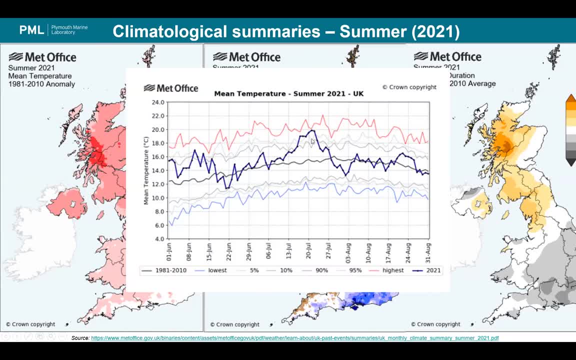 interesting to look at. you can see this, uh, notable possible heat wave that we had in sort of mid to end of july, uh, but then you can almost set your watch by when the schools broke up. this is: this is pretty much around this period that there was again this sudden flip down to um you, 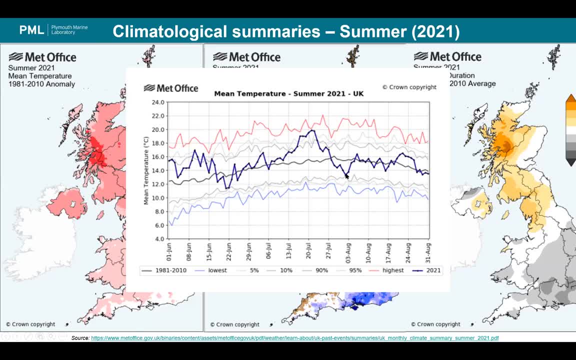 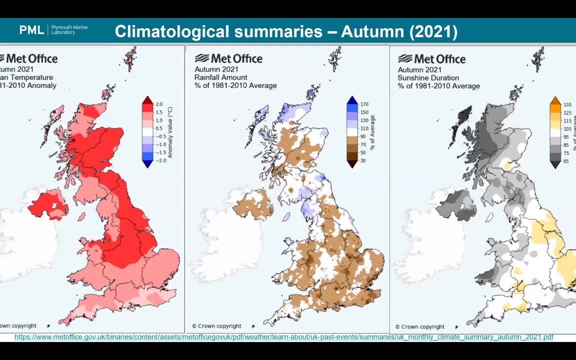 know, colder than average, probably wetter than average, uh, period. so we'll talk about that in a little bit. um, in terms of the storms that we saw this year or last year, autumn again- um, this is mirroring, uh, some of the trends that we're seeing. so we, we found, we find. 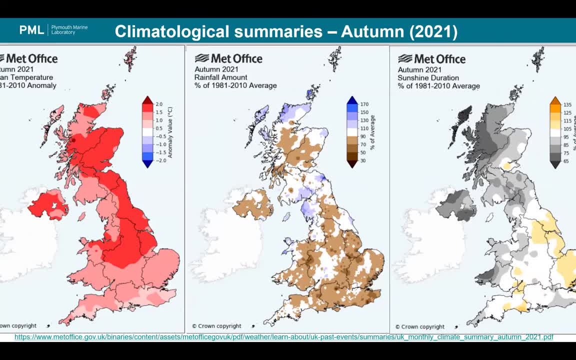 that we've got relatively cold springs, but actually what we're getting are relatively, uh, warm autumns, and- and last year last autumn was no, uh, no different- we were getting somewhere between half and one degree above the anomaly. um, it was not particularly wet or not particularly 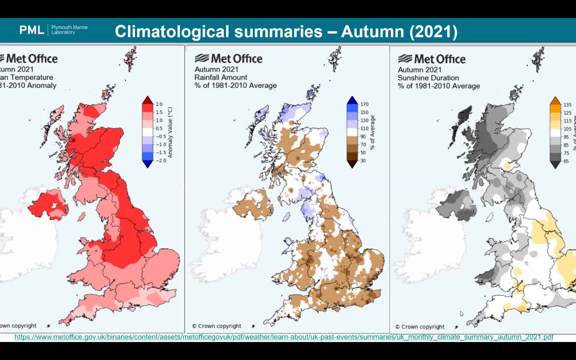 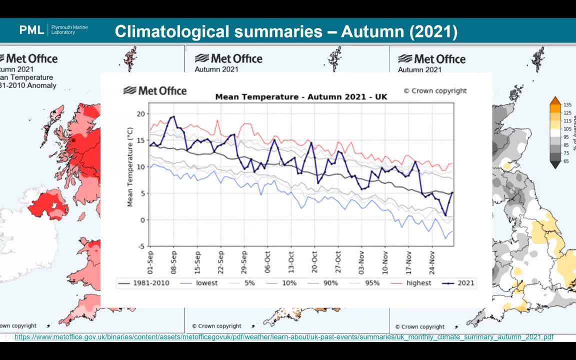 dry. so probably about average rainfall and, uh, and an average in terms of the weather, um, um, in him, um, down at around 15 degrees, and we then measured the overall temperature and the climate. um, at the beginning of the autumn. uh, in terms of, we've got more of a. 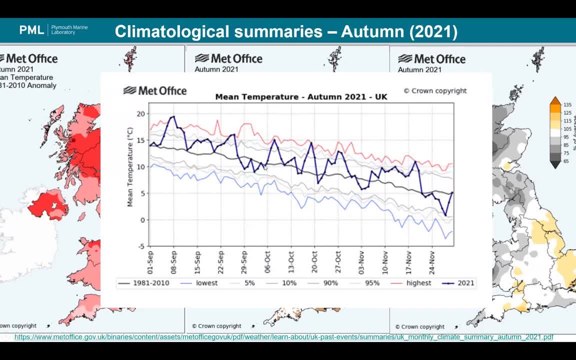 uding and when we went back down here, there was a telling in terms of the uh, the inspiration, and it's not completely right. it's really just to send you a picture in terms of the uh insolation and in terms of the time series. again, you can see that this warmth that we got. 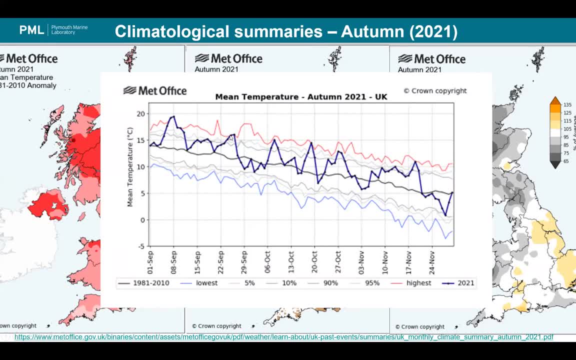 in the autumn was uh. you can see that most of the trace here is well above the uh, the average. in fact, some of the um warmest that have have been recorded in the period um, particularly in early september and late september you were getting these, these warm periods, and it wasn't. 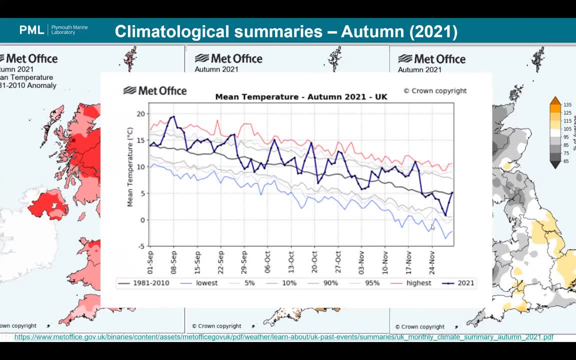 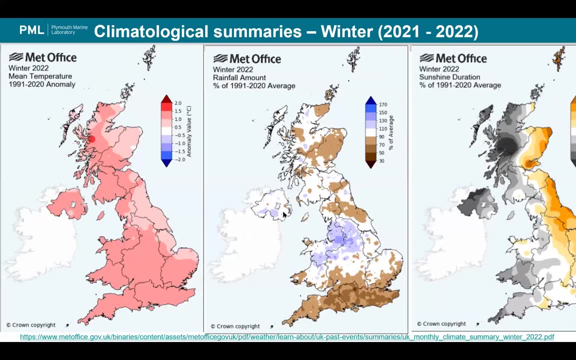 preventive treatment fondation dealing with spartאשoma testicles in the early 20s tends to upper your of November, and this is when storm Arwen came through- that we were getting anything approaching weather that you describe as cold. and then, finally, let's talk about the winter that we've 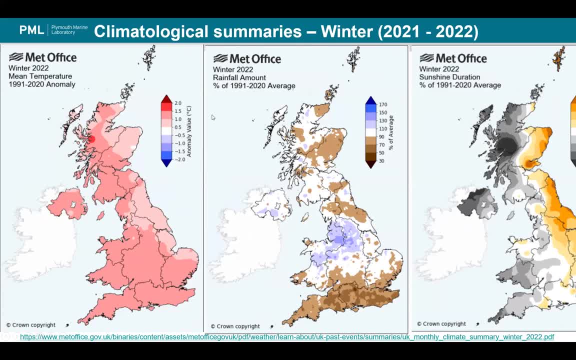 just had. so this is two things to note here. this is winter 2021-22, so December 2021 to February 2022, and you can see now that we've shifted our climatological window, so the climatological window now has shifted to 1991 to 2020 and you can see that the winter as a whole was. 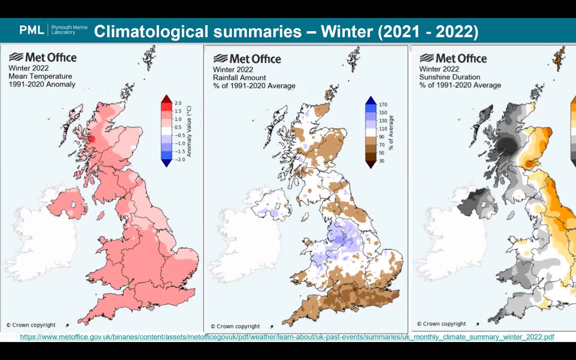 warmer than average and pretty uniformly warmer than average, was pretty much drier, somewhere between 70 and 90 percent of average rainfall this winter, but interestingly was was pretty much duller than average as well. so you get these dull down in the in the west of Cornwall there. 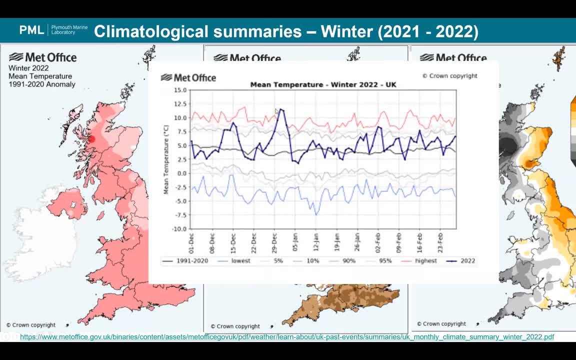 in terms of the temperature, notable warmth, I suppose around New Year. I remember the the headlines in the newspapers was: this was the warmest ever start to a year, and this was born out in the record here. so two notable warm periods, one sort of in early to mid-December. 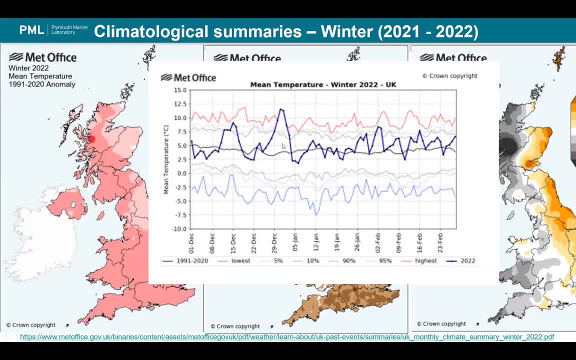 and then this this period in late December, early January, was particularly warm. you're looking at sort of maybe four or five degrees above the average, and that's the central temperature of the year, and that's the central temperature of the year, and that's the central England temperature. so obviously there's some regional variability around that. so enough about. 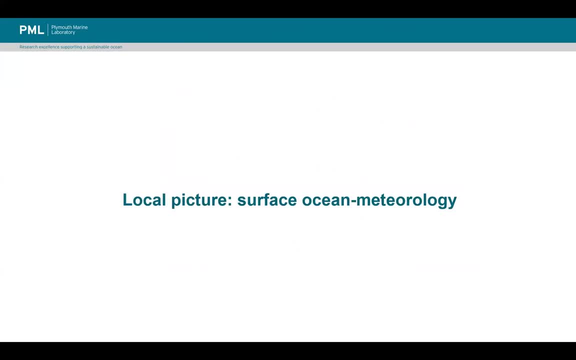 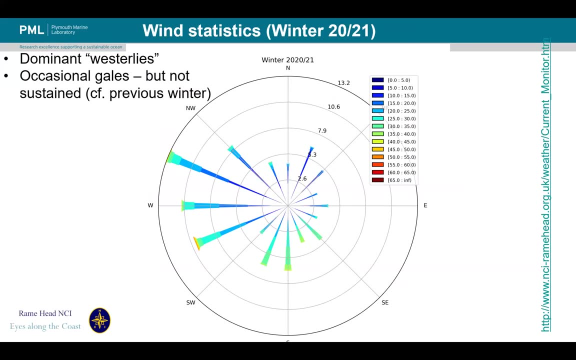 sort of the climatology and and the averages around that. what does this do in terms of the surface ocean meteorology? so what I'm looking at here are the, the the wind direction statistics. so this is for the previous winter, so this is winter 2020 to 21, and this is this plot here. 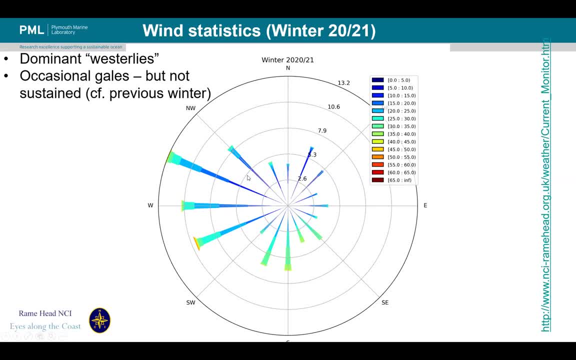 is called a wind rose diagram, and what it attempts to do is it attempts to do is to capture is how dominant wind is from a particular direction. so let's look here. so so the most dominant wind direction, uh, in the winter of 2020 to 21 was something like a west, northwesterly, so 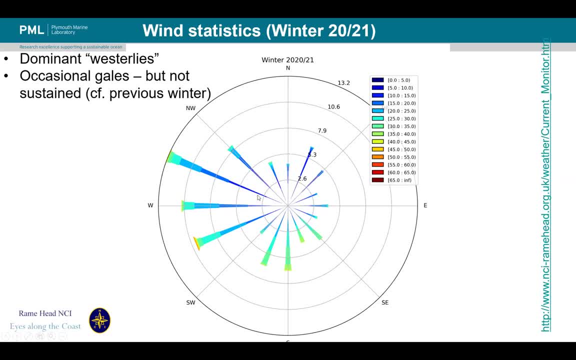 we're getting up to, maybe about 15 percent of the winds were from that direction, and then you can see that the the color gives you how, um, how strong the wind was. so so, basically, our strongest wind direction is from a particular direction. so let's look here. so so, the most dominant wind. 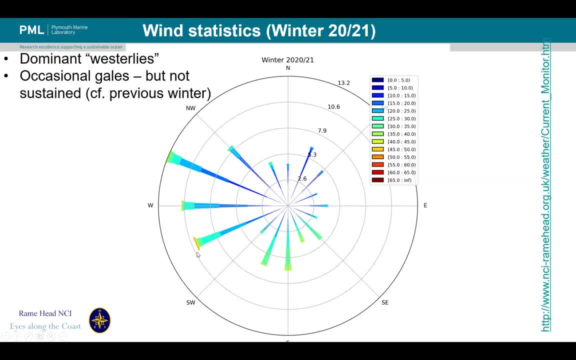 direction is from a particular direction, so we're getting up to maybe about 15 percent of the winds, uh from wind that winter, briefly, uh were sort of on the the in west, southwesterly direction and up to maybe about 50 to 55 knots. so it actually wasn't a particular uh windy, uh winter 2020 to 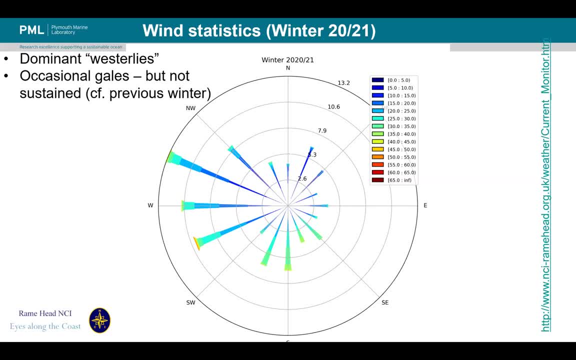 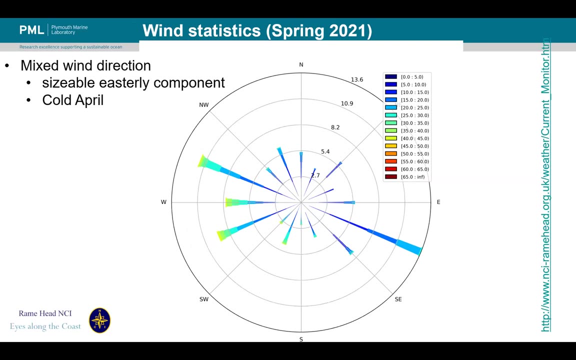 2021. they were occasional gales, but not sustained, so if you remember, um February in 2020 was actually the windiest February on record. we didn't have anything like that uh in uh in last winter or the winter before last, then going into spring 2021. um then you can see. 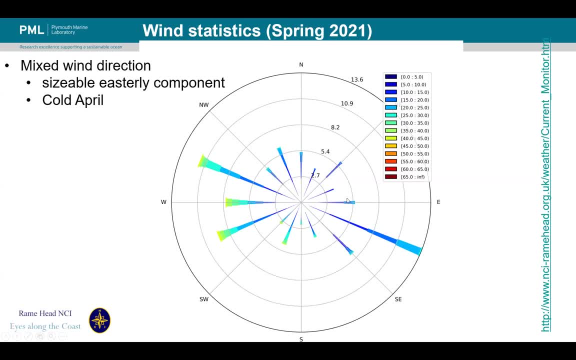 there's been a real shift in the wind direction. um, so what we find here is that this: there is a sizable easterly or east, south easterly component here. this is really um striking, um, not particularly strong, um, so we're only getting wind. uh, wind speeds up to maybe about 30 knots and for a very 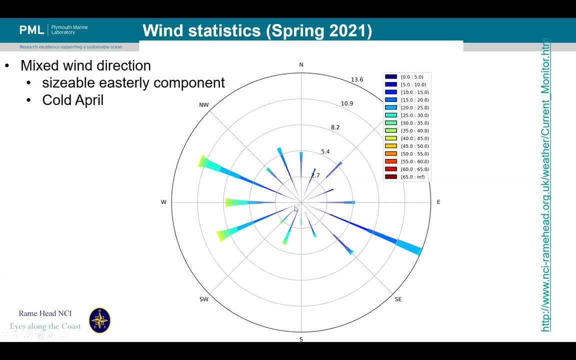 brief period of time, but this could really. this really shows why there was quite a cold um April. uh, last year was because of this direction, uh, of the wind, and then, um, you know, we do still have a westerly component and this is, this is stronger, um, so we're getting up to maybe 35, 40 knots in some of these instances here. 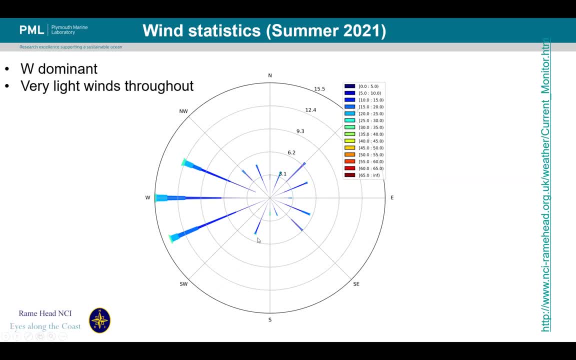 then going through into summer. as you'd expect, the summer is uh much calmer, much less in the way of gales, pretty much um. again, there's a dominance of the wind in the west, south, westerly component and westerly uh wind type uh, but very light winds uh throughout. uh light and variable winds, I would. 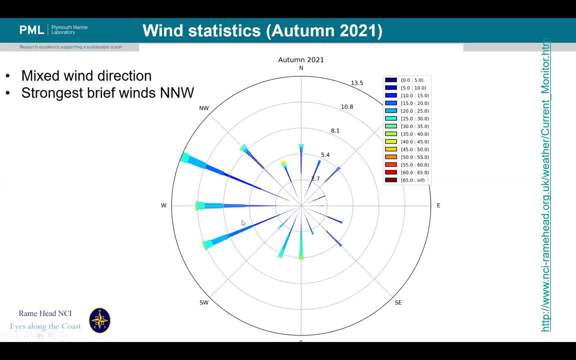 say, is best way of describing, uh, summer 2021, and then there's a very much a mixed wind direction in autumn 2021 and I'd just like to draw your attention to this- the strongest winds in this period, unusually where it was a north, north, westerly, so I'm guessing this is the fingerprint. 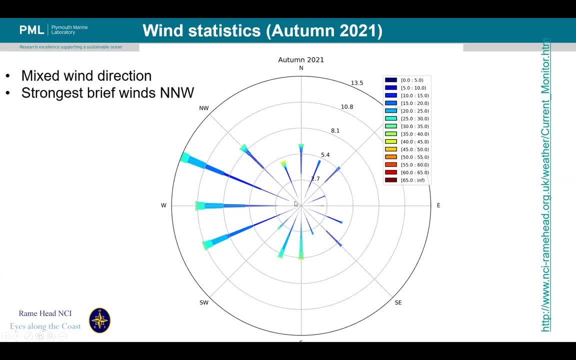 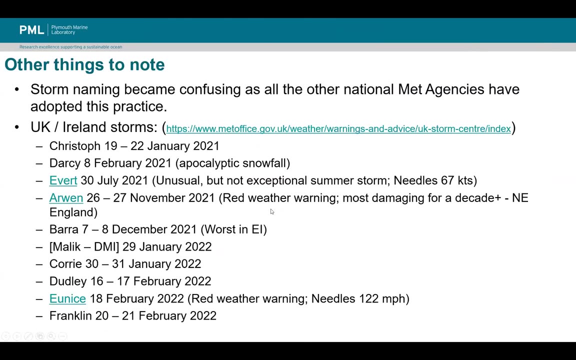 of um storm almond. we'll talk a little bit about that one in a moment. uh, very uh, brief wind, uh, strong winds from that direction, but again a pretty mixed picture in terms of the wind uh direction. so, um, I'll take you through the named storms of uh 2021, uh and into early 2022. 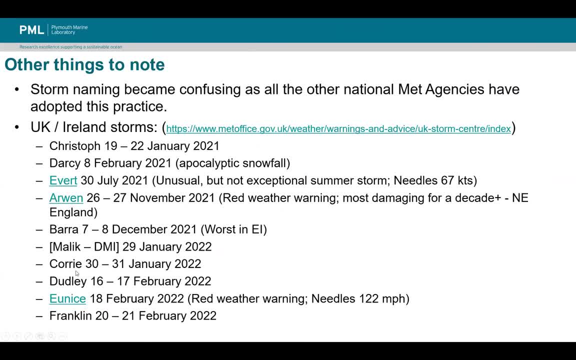 because it actually starts getting a bit more interesting in 2022. um, so these are the named storms by the UK and Ireland, uh Met Office. um, the UK and Ireland Met Office started naming storms, I think in about 2015.. um, but then all the other Met agencies in Europe decided this was a really good idea. 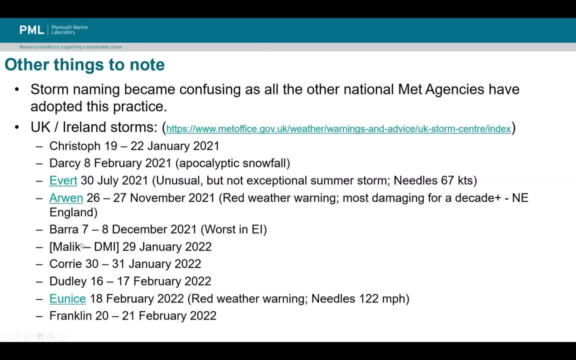 and then that really made things very confusing in terms of following uh, storm naming um, so I've highlighted one down here which which could be important. so, uh, the first name storm of- uh, that or or of 2021 was Christoph, so that would have been the third one in the in the series. so, 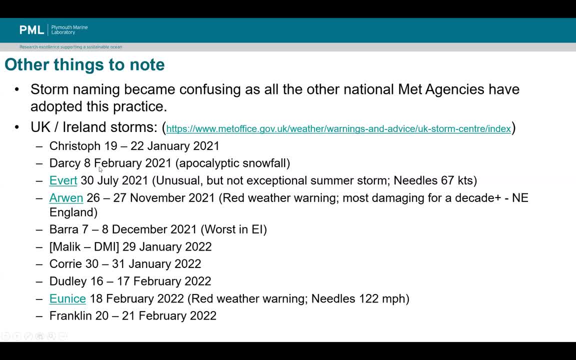 Kristof was between the 19th to the 22nd of January, Darcy. there was a forecast to be apocalyptic snowfall, but that actually never rocked up. I think it was a little bit snowy in the in the east of the country and into the near continent, And then this one's quite interesting. 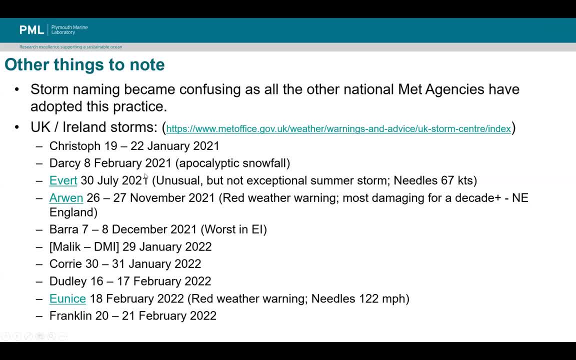 so Storm Evert. This is unusual, but it wasn't exceptional in terms of a summer storm, but you can see how late in the season. there wasn't anything in terms of named storms after the 8th of February and there wasn't one until the 30th of July, and actually that's almost. 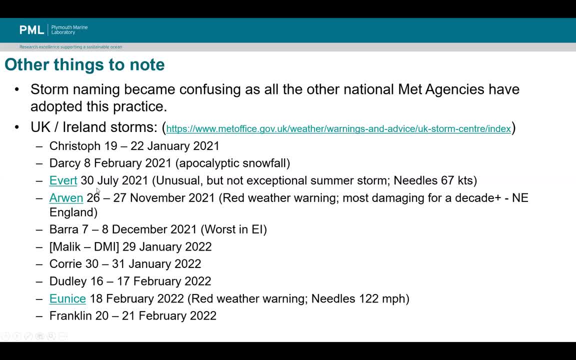 the very end of the year, So they start naming the storms in about September: Storm Arwen. So they restarted the alphabet again, So Arwen was particularly noticeable. There was a red weather warning for the northeast of Scotland and England. This is one of the most damaging. 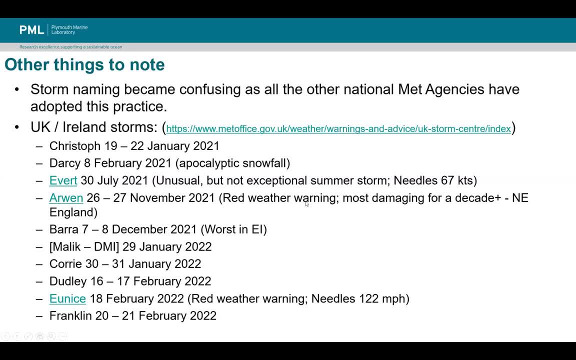 storms for a decade. There was quite a bit of snow associated with the tail end of it And there was quite a bit of damage done to infrastructure, power lines etc. in the northeast of England that took a few weeks to really sort out. 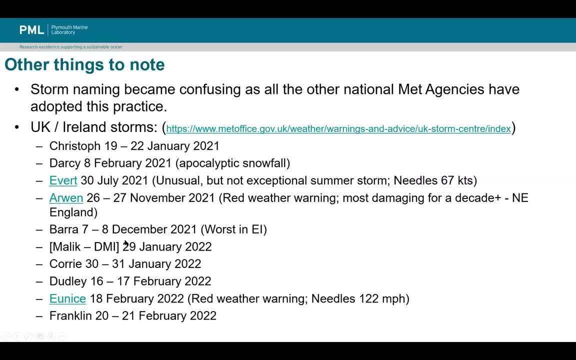 Then there was Storm Barra, on the 7th to the 8th of December. This is worst in the Republic of Ireland. And then this is where it gets confusing. The Danish Met service named this Storm Malik, which came through on the 29th of January. Corrie, which hit us more on the 30th to the 31st. 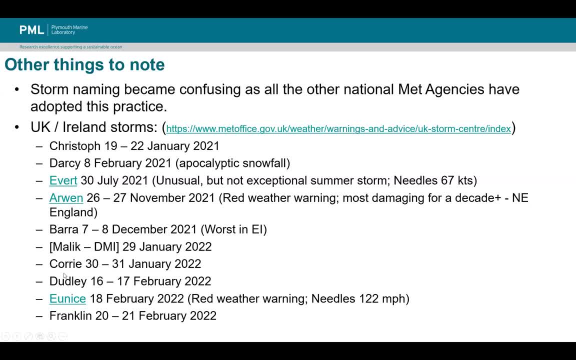 And then there was this trinity of really fairly severe storms. particularly Eunice was a notable storm, probably the worst for about 30 years, probably since the Burns Night storm of 1990.. We had a red weather warning down here, if you remember rightly, and the highest wind gust. 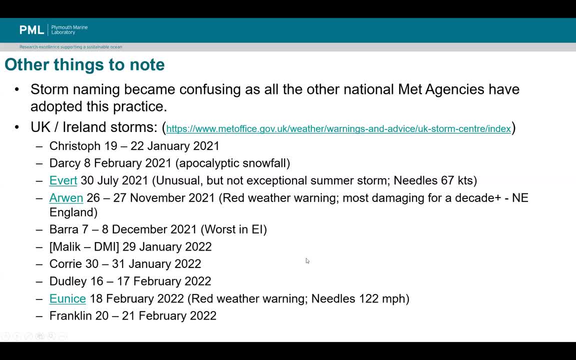 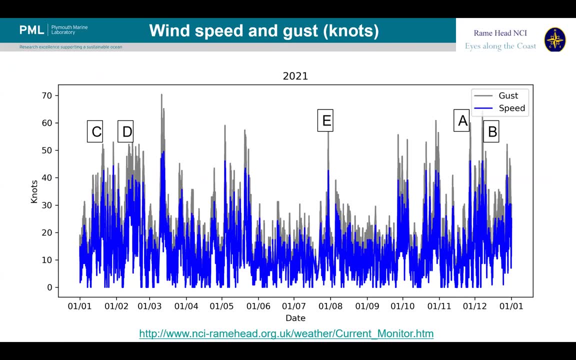 was at the needles of 122 miles an hour. I'll show you some of the observations we got. And then, And then, pretty much on the hot, hot hot, on the heels of Eunice, we had storm Franklin. So what did this look like in terms of the, the wind speeds that we measured at rain head? 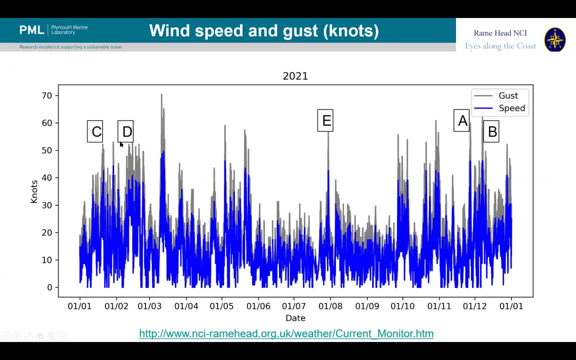 So you can see the name storms here. this is Christoph in C Darcy in D, Everett. so this was this unusual, so we're here through into into August or late July, early August. this is the storm Everett, so wind gusts up to about 55 knots. 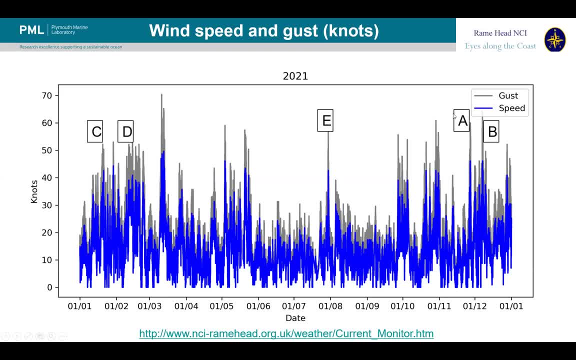 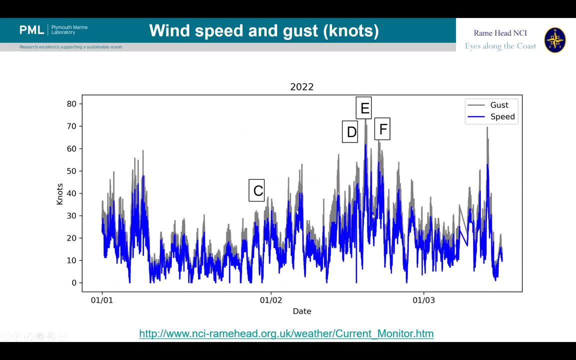 So certainly enough to blow a tent away. and then storm Arwen, which didn't affect us quite so badly down here in the southwest, and storm Barra, And then, in terms of what has happened during 2022, we can see this, this trinity of storms. 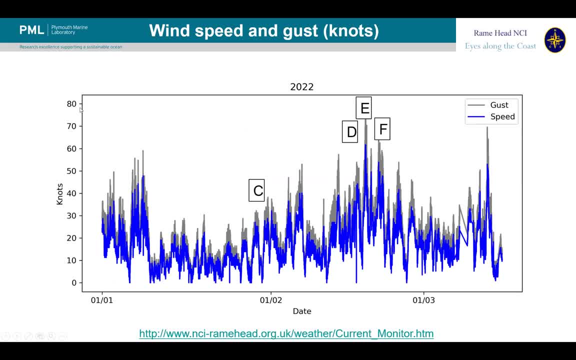 I've changed the scale here so this is up, up and over 80 knots. so sustained winds of over 60 knots is hurricane force on the Beaufort scale. So you can see that certainly Eunice gave us sustained winds over over hurricane force. 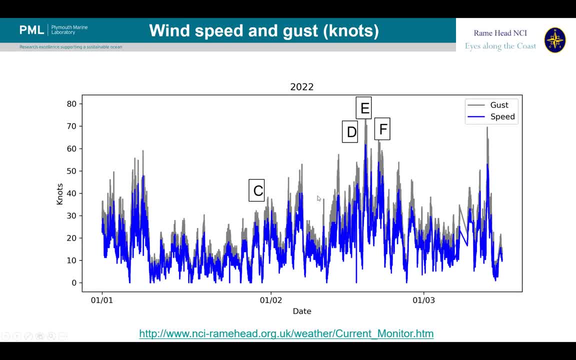 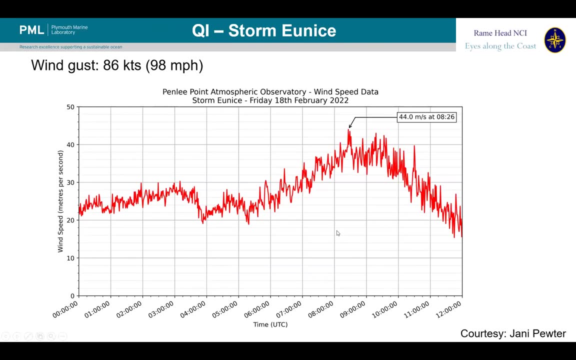 for a brief period. So that's the other thing to note is really that the that there are, that only really this storm Corrie didn't really hit us very much at all down here in the southwest, And thanks to Yanni-Puter for this, this plot here. this these are the data from storm Eunice. 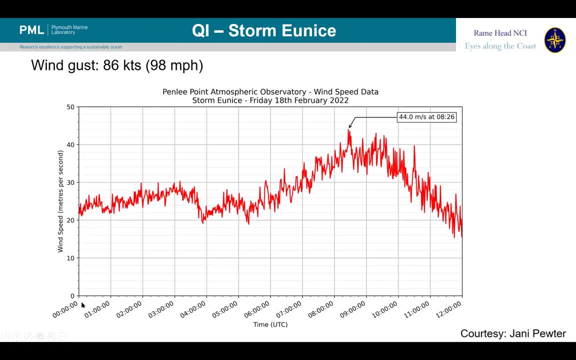 for the 18th. So Friday, the 18th of February, And then we've got this, And then we've got this. So Friday, the 18th of February, going through from midnight to to 12 o'clock, which is. 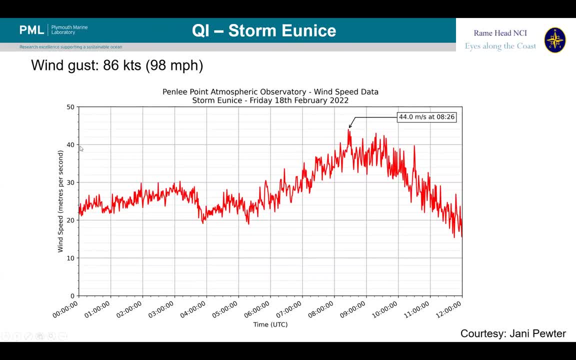 when the storm had already passed And you can see this is. this is wind speed in meters per second now. so we'll have to do a very quick mental, or a bit of mental, arithmetic. and the the highest wind gusts that we recorded at Penley point was 44 meters per second half past eight in the morning. 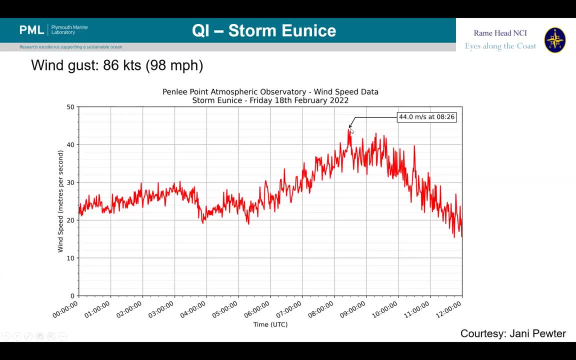 which was actually when most of the damage was done in this, in this storm, which was actually when most of the damage was done in this, in this storm. It was around it. so that's around about 86 knots or 98 miles per hour. so we're still. 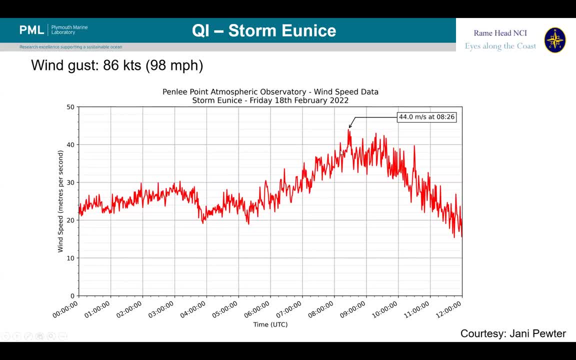 about 20 miles per hour less than what was recorded at the needles. You can see that pretty much the storm was was enveloped in over a period of about two hours. before then the wind drops very no spillway between 1010 o'clock in the morning. 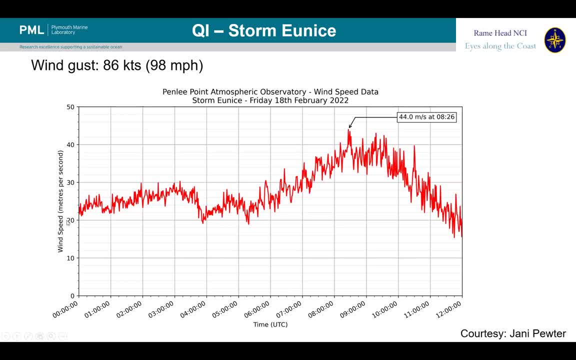 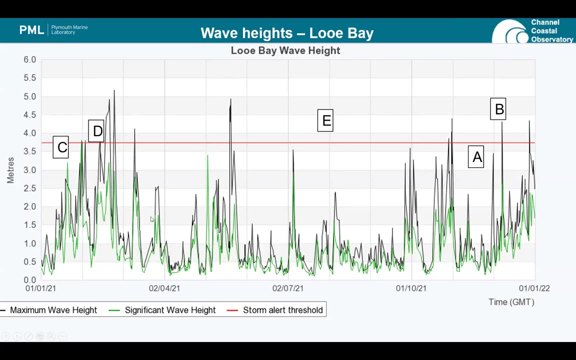 and midday, But even this is still gale force. so you know, it was pretty, pretty sustained winds for Around about 12 hours or so, And then in terms of what happened, to the wave heights. so this is what the you know. 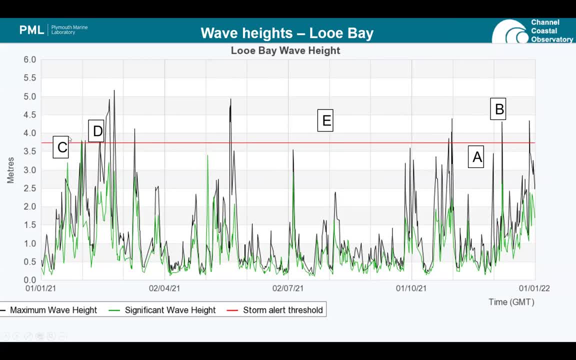 the impact, the noticeable impact, of these storms on on the waist height. so again, this is January 2021.. This is April, July, October and through to January 2022, so this is last year. looking at the wave heights, a storm threshold is set. 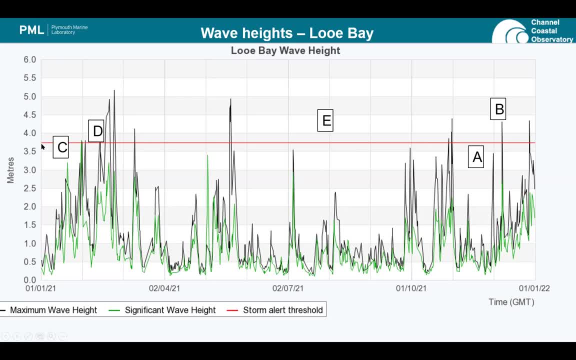 Lou as a significant one. So you can actually see that a lot of these storms, these named storms, didn't really have a huge impact in terms of the of how, how large the waves were. in actual fact, it's probably some of the sort of the more deep ocean swells that are giving us that the highest when the 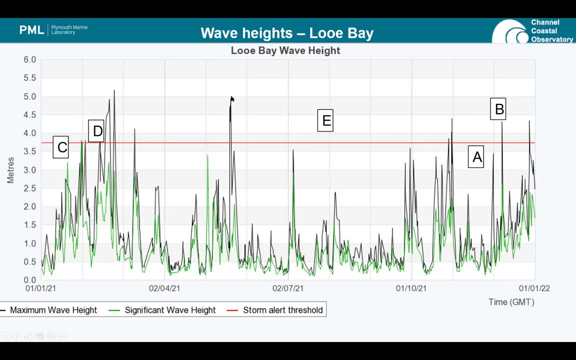 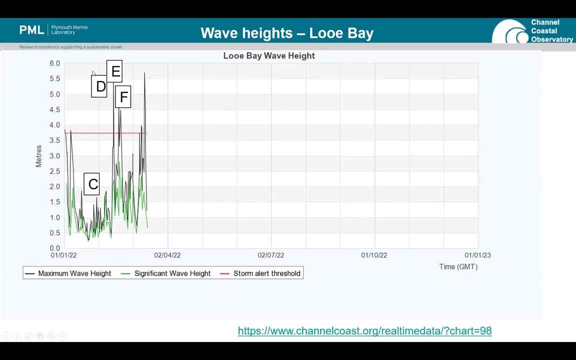 highest waves, so up to about five meters here in in May 2021.. And you can see that, you know that, Although They're not named, there are some interesting events that happened earlier in the period. and then this is the trinity of storms that came through in in in February, so storm. 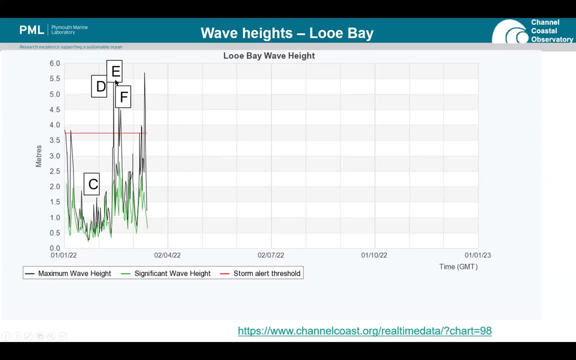 Dudley units. so we got, maybe when wave heights over five and a half meters in Lou Bay before it dropped away very, very quickly. This is interesting to know. I think you know these deep ocean swells that we're getting coming through and being picked up by the Lou Bay. 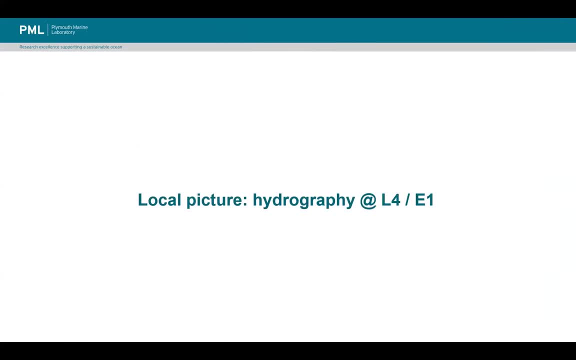 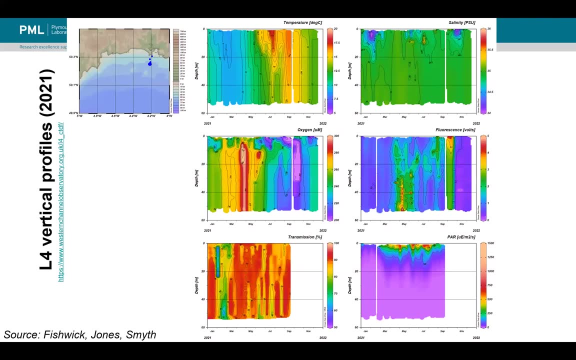 Boy, There's no name storms associated with them. So what did that then mean for the hydrography at L4 and E1.. So this, this here is the, the. this is the vertical profile that we measure with the quest. so this is depth, so zero, down to about 50 meters at L4, and things to note. 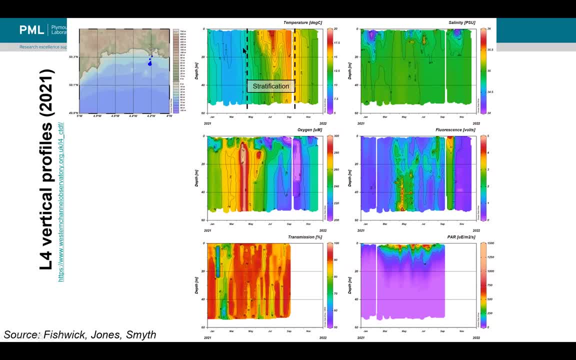 This is the period of stratification. so stratification was fairly late in starting In in 2021. So this is the period of stratification In 2021, sort of started in early May and didn't really get going properly until June. 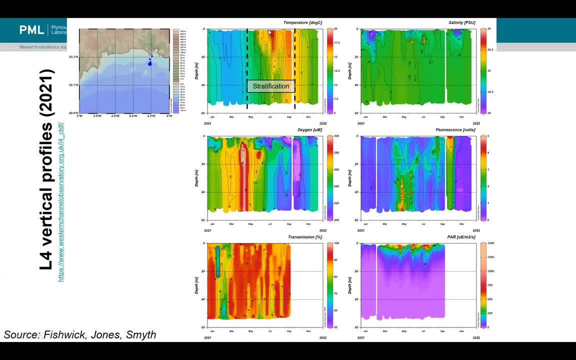 You can see the notable warm period here in terms of the higher temperatures, so temperatures of 17, half 18 degrees in the surface layer and you can see this very marked stratification. so it's about 17 and a half degrees surface back, 1415 degrees lower down about 40- 50 meters. 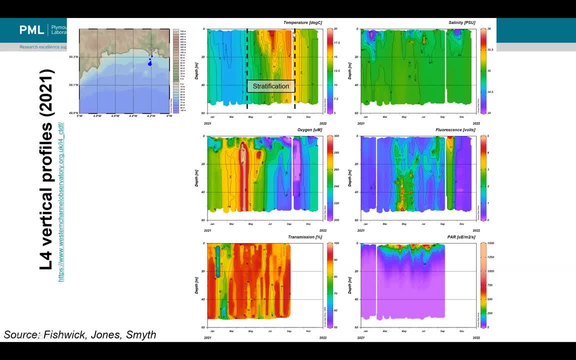 down in the water column And then stratification itself Broke down in probably late September. The data from the latter period we we thank the, the MBA CPS, for coming to our rescue. so we had real engine problems with the question that time. so we've got brand new engine on. 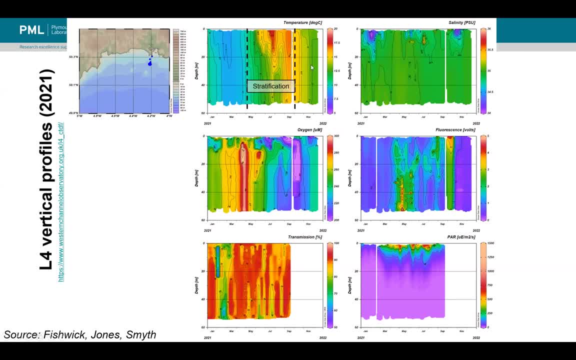 quest, But this is data taken by the sepia And you can also see in the salinity signature. This is very typical of what we'd see in the wintertime. so what we see is when, when it rains A lot. 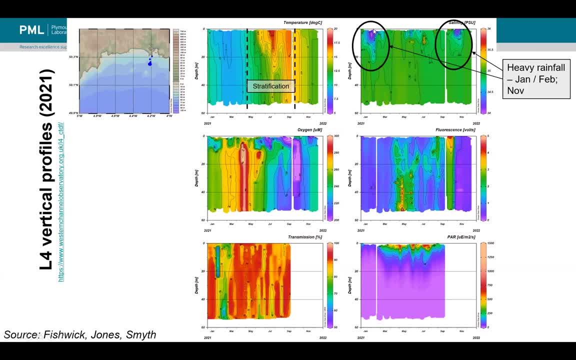 And there's a, there's this heavy rainfall but then flushes down through the Tamar. you see these lenses of much fresher water. so fresh water we mean sort of about half to maybe a whole salinity unit lower than you'd expect, and we saw that sort of in in January. 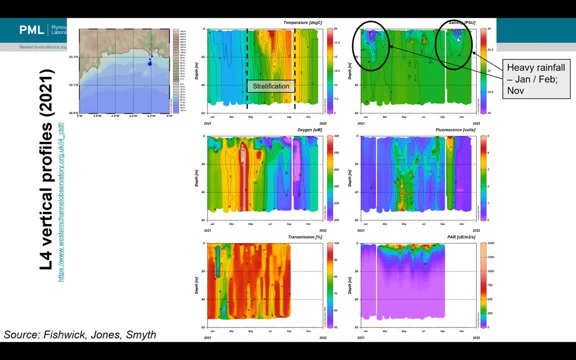 through into February and then sort of again. we saw that in November And then there was a late spring boom last year, so it was sort of into the middle of April or the end of of April before anything started going, But then in terms of the summer and the autumn blooms. so it seemed to be a couple of episodes. 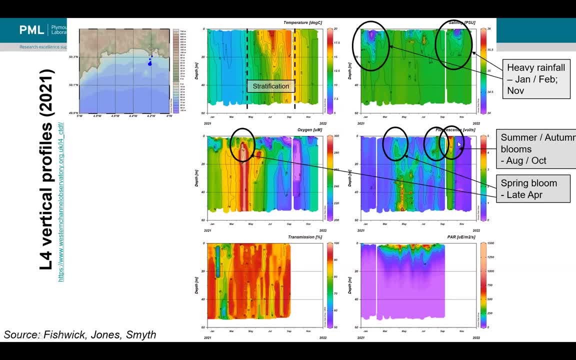 of summer and autumn blooms here in the record. Sorry, I should have pointed out this is fluorescence, So that's a proxy for the chlorophyll concentration And this is oxygen here. so you can see sort of how oxygen and fluorescence work. And this is a proxy for chlorophyll concentration. 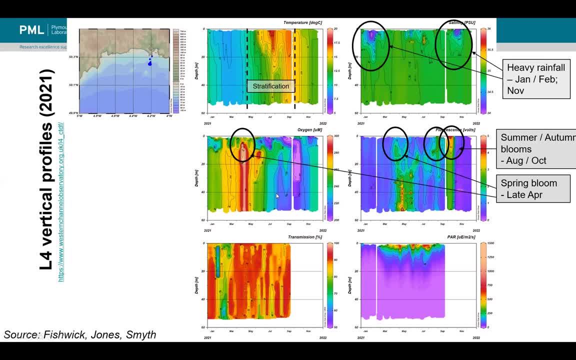 And this is oxygen here, so you can see sort of how oxygen and fluorescence work. And this is a proxy for chlorophyll concentration And this is oxygen here, so you can see sort of how oxygen and fluorescence work. And this is oxygen here, so you can see sort of how oxygen and fluorescence and fluorescence. 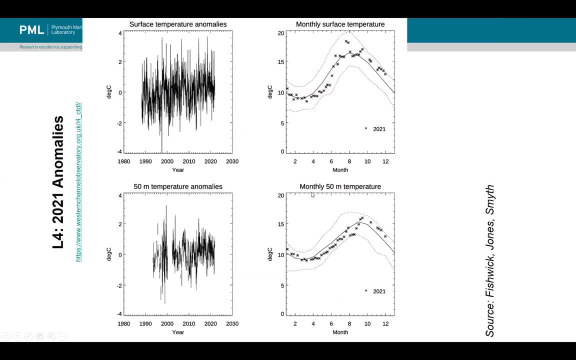 relate to one another here because of the phytoplankton activity And then in terms of what this looks like in terms of the anomalies. So what we've done here is this is a surface temperature anomaly in the top left and then the 50 meter temperature anomaly here in the bottom right. 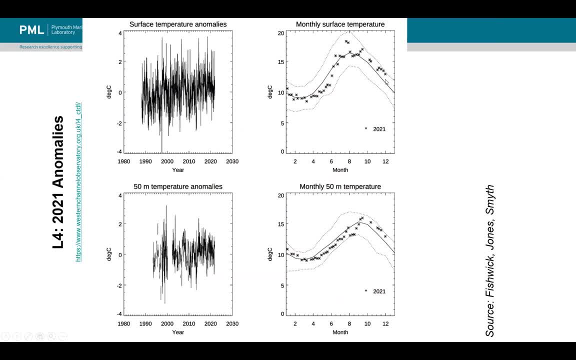 And then you can see every weekly sample that we made during 2021 and how that sits against the the average. So this is the average monthly average as you go through the year. so generally we'd expect the coldest time of year is about now, sort of early March. then we get temperatures at L4, typically down to about. 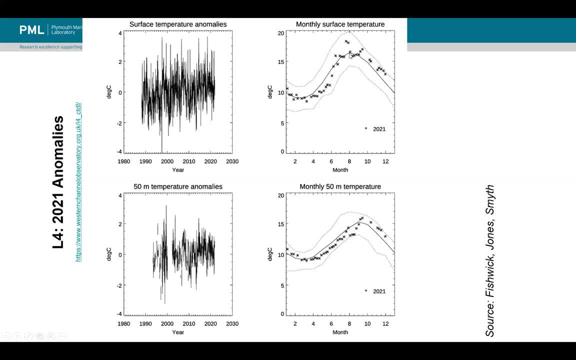 just under nine degrees and then up in the surface layer up to about 16 degrees in the summer. and then you can see what happened in 2021. again, you can see this colder spring period, and it's not just at the surface. you can see that cold spring weather. it's all the way down to 50. 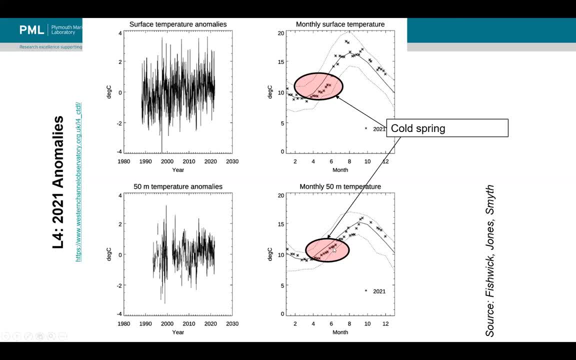 meters down in the water column, so maybe about half a degree at 50 meters, maybe a whole degree, maybe two degrees colder than average in 2021 spring, and then you can see this July warmth. what happens? the water column responds pretty quickly, or the surface of 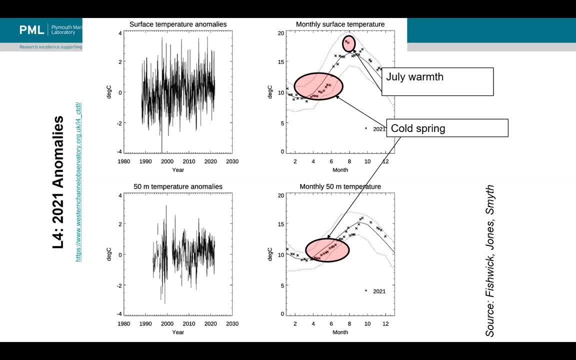 the water column responds very quickly to any warmth and you can see that here in the surface and then you can see then the stratification breakdown which is then when the top of the water column and the bottom of the water column the same temperature. what does that look? what? 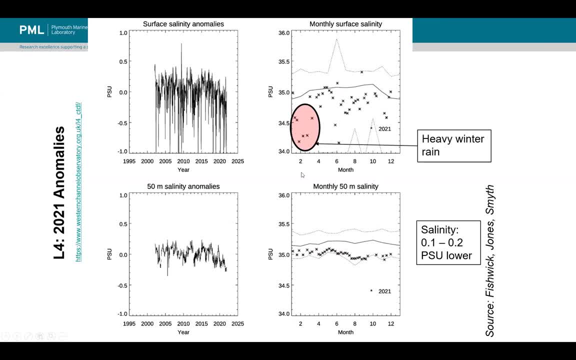 does it look like in terms of salinity? well, again, you can see these pulses of colder- sorry, of less saline, fresher water at the surface here, these lenses and how this looks like in terms of anomalies, and then you can see this drift downwards in terms of the average salinity. 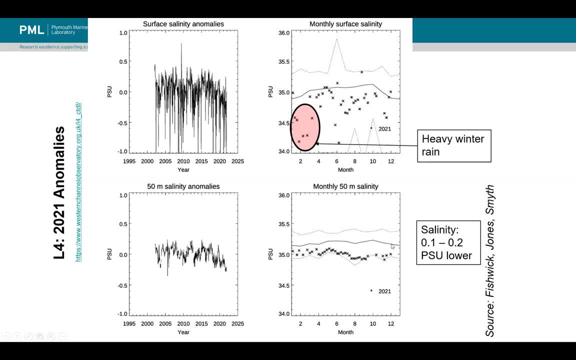 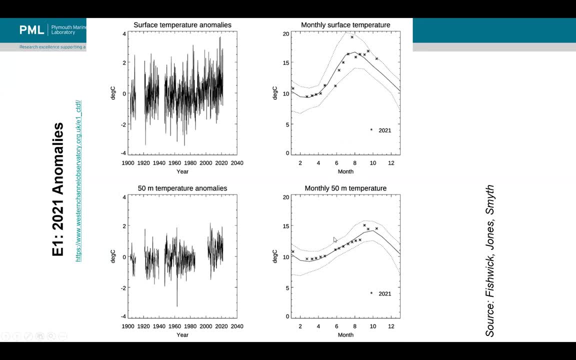 over the last year. so we've got progressively fresher. we need to look into mechanisms of why that's the case at the moment. and then let's look at E1. so E1's got a much longer temperature and salinity time series- one of the longest time series in the world. 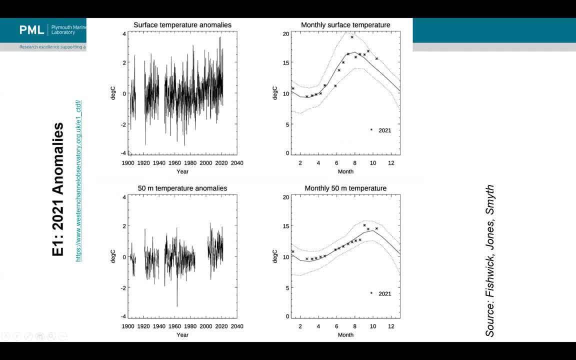 maintained by NBA and PML. so this goes back to 1903. so you can see the beginning of the time series here, with the breaks for the world wars and the anonymous. so you can see that there's this period of warming over the last maybe 35, 40 years now. 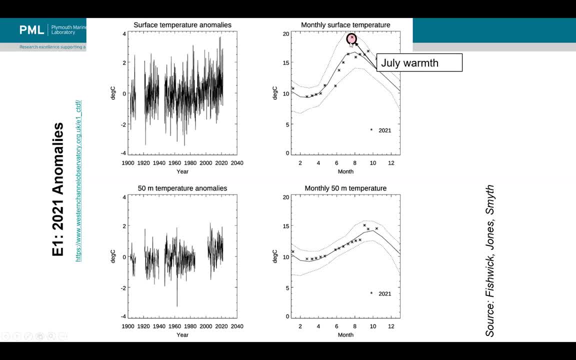 and what you can see in the series again for for E1 you can see this this July warmth and you can again see the stratification breakdown. we only visit E1 typically in the summer, every fortnight or so, and even less frequently, maybe once a month or so in the in the winter time. 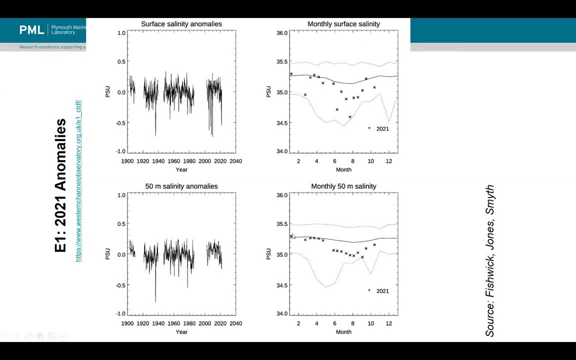 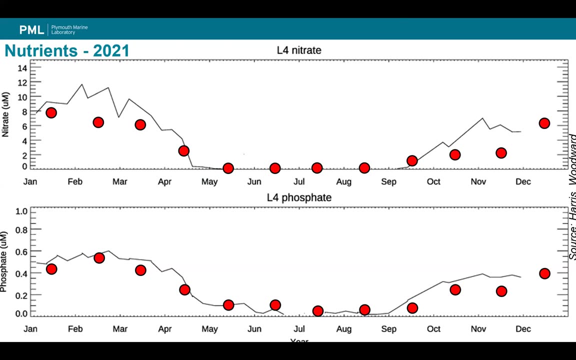 and again this: this shows that there's this general downward salinity drift at the moment. but you know this. there's no reason to to believe that this is a long-term trend and then finally just finish up with the what the nutrients have been doing at L4 over the past year. so thanks to Mount Woodward and Carolyn Harris for these data. so what we're? 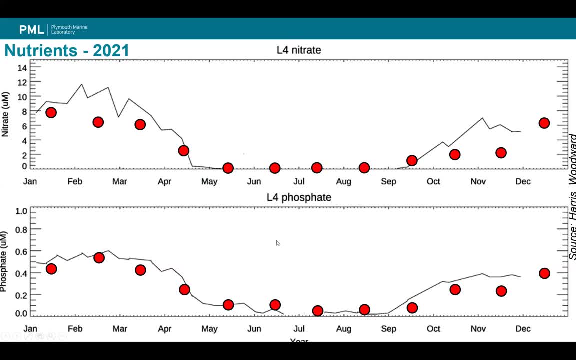 showing here is the nitrate, the surface nitrate at L4 and the surface phosphate. so these are key inorganic nutrients in the ecosystem, and what you can see is the red dots are your average levels of nitrate and phosphate for each month, and then the actual measurements that we took in 2021 are this: 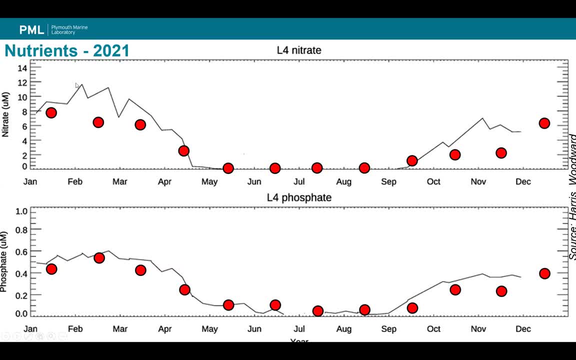 the solid line here and you can see that last winter there was probably about- I don't know- two, two to four micromolar of nitrate, more than you'd expect on average. and then you can see during the summer what happens is here. is that the? 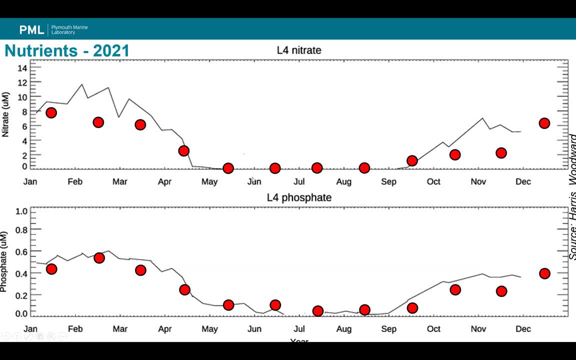 nitrogen basically finishes up all the all the nitrate in the surface. so that's why the bloom crashes after just after the spring bloom in the surface because it's nitrate limited. phosphate never becomes limited at L4, but obviously there's a there is a seasonal cycle, so we generally would. 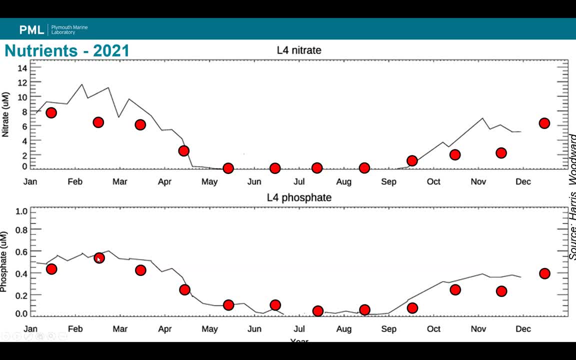 measure around about 0.5, 0.6 micromolar in the winter time and sort of down to about just over or just about measurable um in the surface in the summer time. so on that note I will stop my presentation, and I think that's. 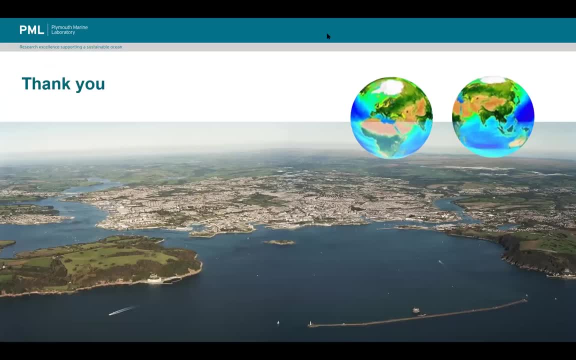 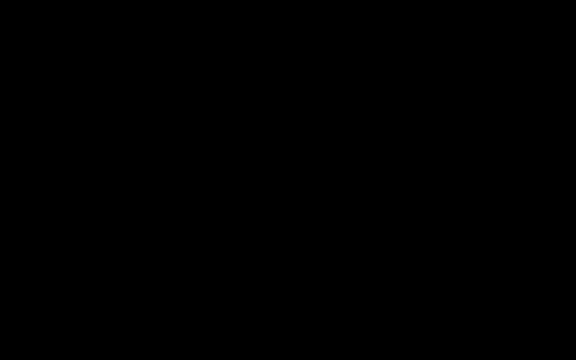 all I've got. yep, that's all I've got, so I shall stop sharing there and hand back over to you Keith. thank you very much indeed, Tim. all fascinating stuff, um, especially the comparisons over the years. um, I've only got one bit of chat that I've picked up um, and that's. I'm looking for it now. 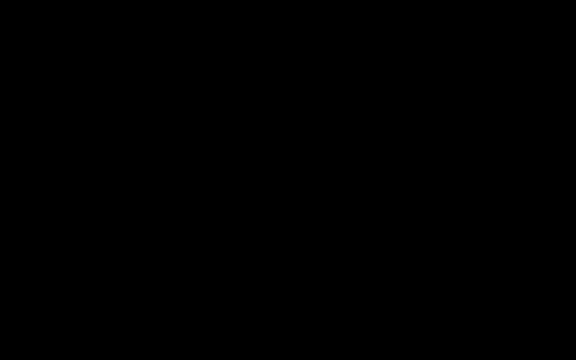 sorry, I'm not able to shine that up. uh, oh, it's from um. your Johnson isn't 44 miles per second hurricane force? yes, so I think I believe that that's 44 meters per second, meters, not miles, yes, so yeah, well, it's all these these units around um. thank you for that question brought uh, so 65. 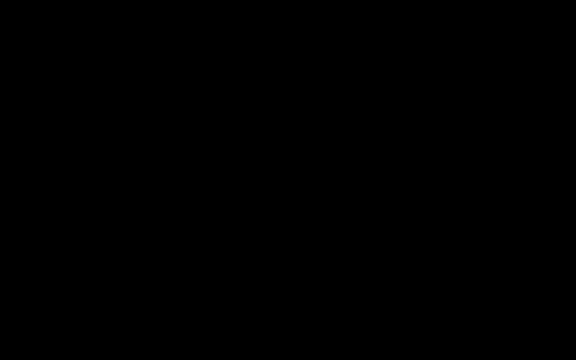 or 60 to 65 knots. sustained is is hurricane force Beaufort scale 12: um 44 meters per second. I think we put there was um I can't remember how many, how many knots it was. was it 98 knots or 88, not something like that? so 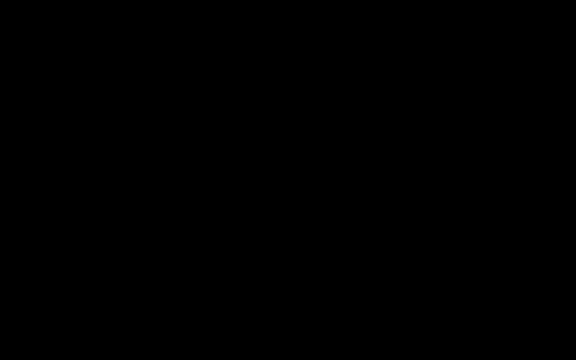 it's well over hurricane force, but that's just the gust, so we need to be careful when we look at these things. the really damaging thing to note is actually when you've got a wind speed of 80 mile or 80 knots, it's twice. it gives you twice the amount of force. as great you mean, it's. 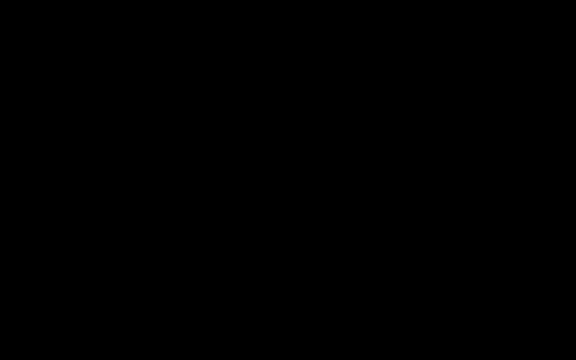 as one that's of 60 knots. so just by increasing that amount, that's what does the real damage. um. so that's, that was just something that i i picked up on um during that particular storm. thank you very much indeed again. tim um participants, if you have got uh. 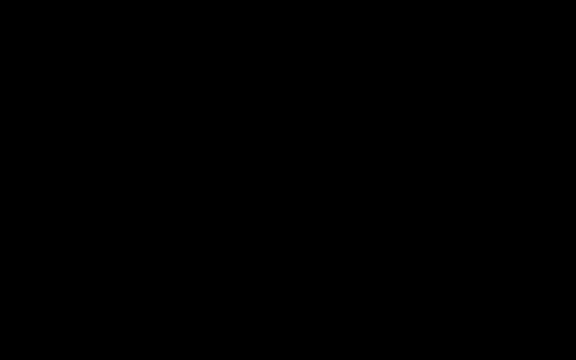 questions? uh best to put them in the q a um, but i'm monitoring both q a and chat and, of course, if you put a question in q a and somebody else can answer it, you know, do answer it, otherwise i'll pass them on to the uh panelists, um. so thank you, tim. 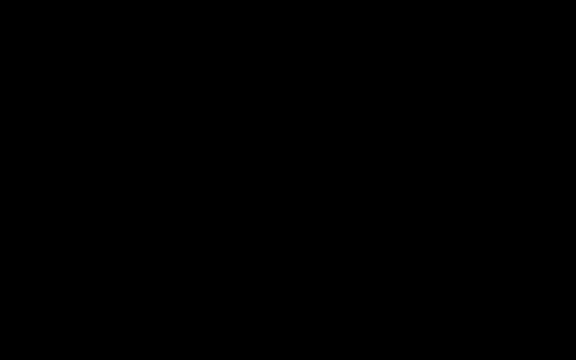 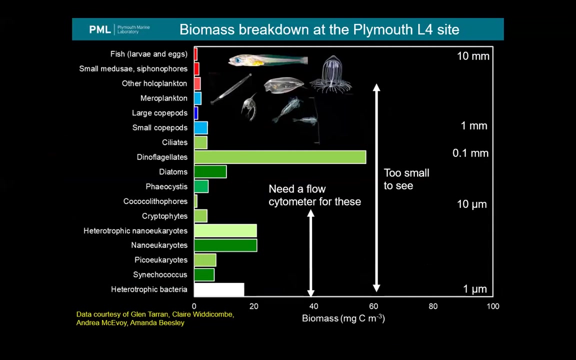 uh, we're now ready to move on to angus atkinson, to uh talk about plankton. uh, during 2021. so over to you, angus. okay, thanks very much, keith. i'll just share my screen now. thank you right. can everybody see the um screen in presenter mode? 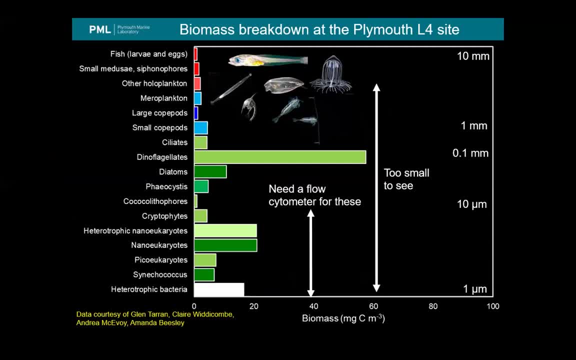 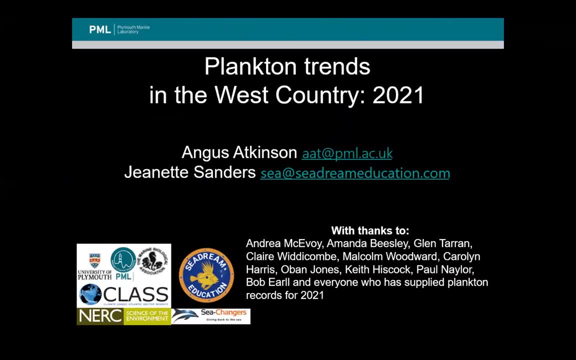 that all looks fine. that's good, right, um so? um, i'll just go back to the beginning. i don't know how it got to there, so you've had a sneak preview, but, um, this is a joint presentation. i'm going to be sharing it with jeanette sanders, who's going to present four slides in the middle. 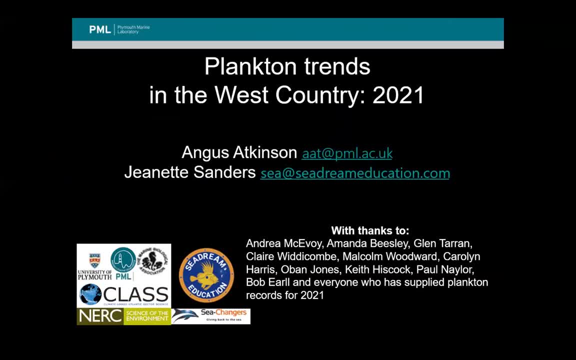 of this presentation on the southwest jellyfish survey. but before i start i just want to thank colleagues at pml for supplying large amounts of time series data, um on the plankton and also from some of the southwest marine ecosystems organizers, as well as um basically everybody who supplied plankton records for last year. 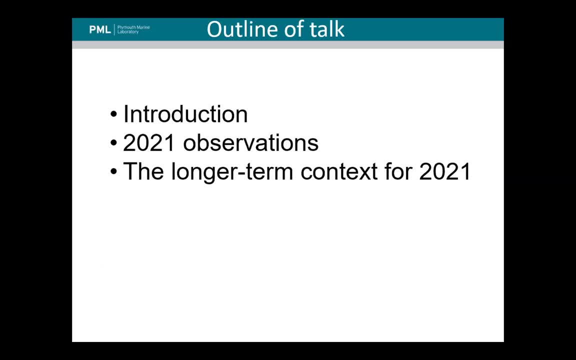 so the structure of the talk. i'm going to present half a dozen slides just to introduce West Country plankton and plankton food chains. then the main part is the observations for last year and placing them into the longer term context of time trends for over the last 30 years or so. 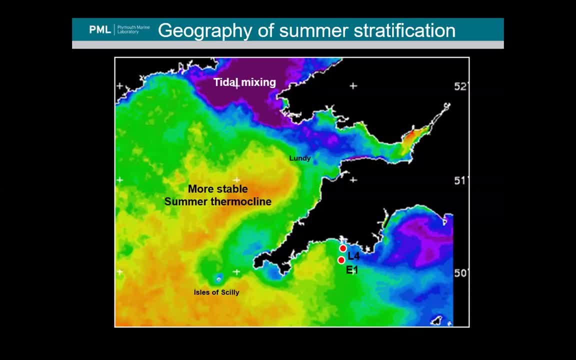 So this is a slide I showed actually last year and it sets the L4 and E1 sites that Tim has just been talking about, sets them into a sort of wider scale context and that's a heat map of surface temperatures from satellite records. So the warm yellows and oranges are the warm. 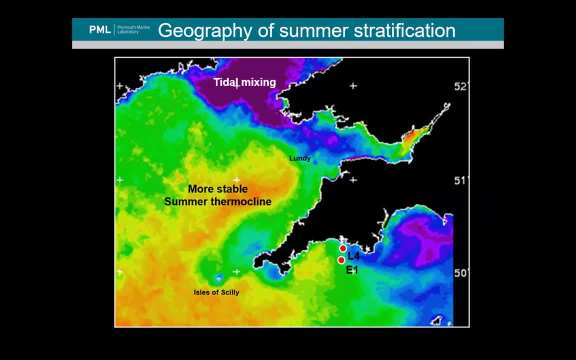 stratified surface water that heats up in the summer and it is insulated from the waters underneath and it runs out of nutrients and that's separated from more tidally mixed areas, often in shore, Which are those blues and purples, which are cooler water, more nutrient rich. So there's quite a big. 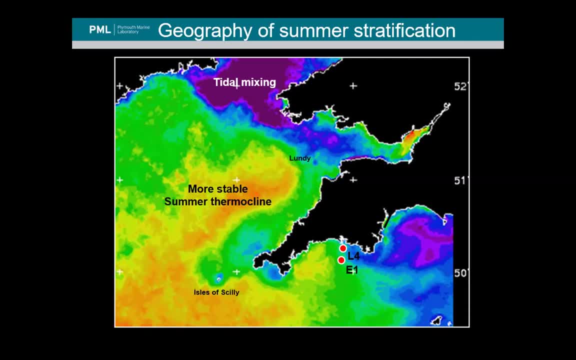 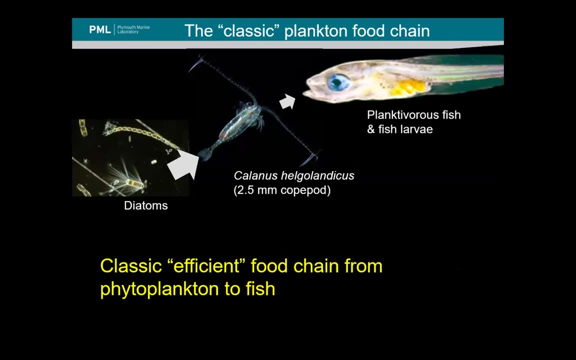 diversity of habitats in the West Country And the classic plankton food chain that you'd get in a textbook is where the phytoplankton, which I've illustrated here by diatoms, the primary producers, are eaten by the zooplankton and I've illustrated them. 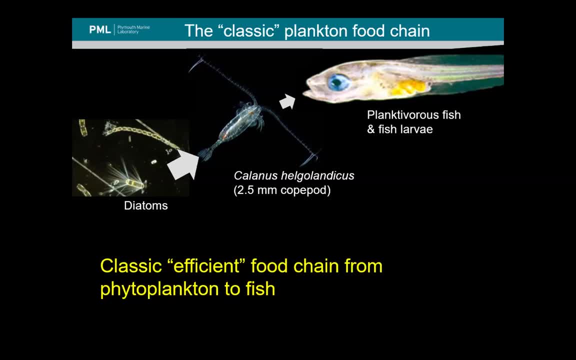 by Calanus helgolandica, One of the biomass dominant large zooplankton, and they're in turn eaten by planktivorous fish such as herring and sprat and pilchard, or by the larvae of demersal fish. 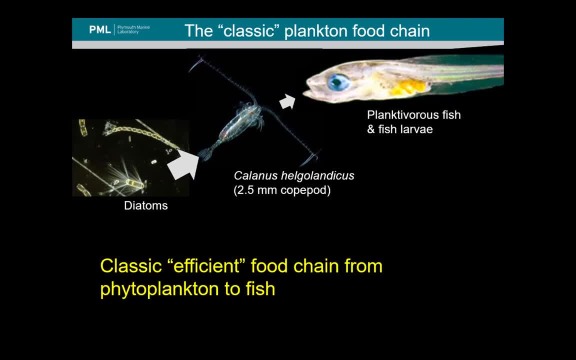 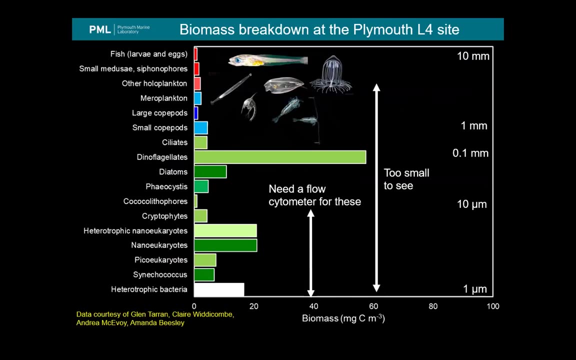 So that's the sort of classic textbook picture of the food chain which I want to keep in your head because I'm going to return to it later in the presentation. So this is actually a biomass breakdown of all of the plankton that we sample at the L4 site, and I've ranked these. 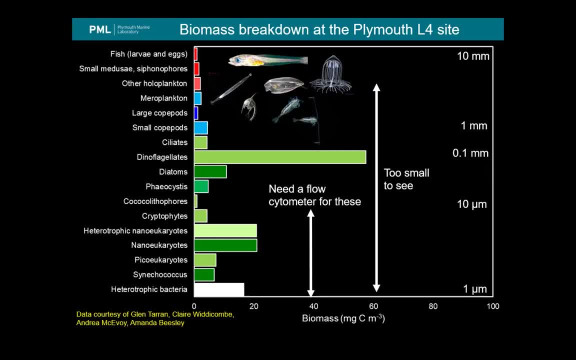 sort of groups. we call them functional groups or broad taxa. I've ranked them from the largest at the top: the fish larvae and the eggs of fish through the jellies, various plankton, right down to heterotrophic bacteria about a micron long. 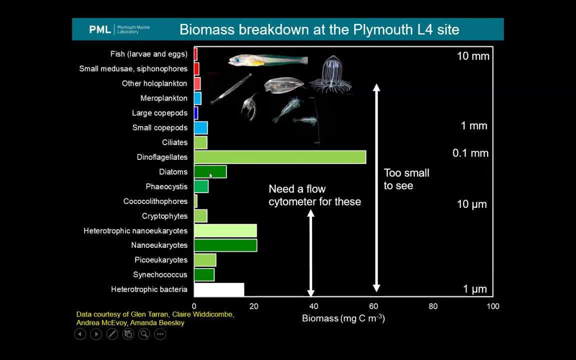 So let's have a look at the image. So if you- I don't know if you can see my cursor, but I just described this classical food chain, The diatoms- they're actually quite a minor proportion of the total biomass. In turn, the large copepods, for example, the calanus, a minor proportion, as are the fish larvae. 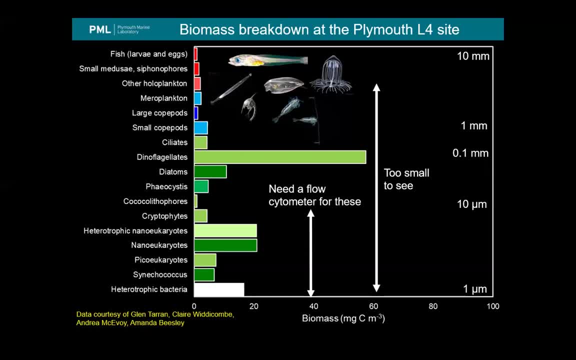 So a lot of the plankton that you see are right up this top end and they're a tiny proportion of the biomass. Most of them you need either a microscope to identify or they're even too small for a microscope. You need a flow cytometer. I've colour coded the basic sort of trophic levels so that you can see the various phytoplankton. 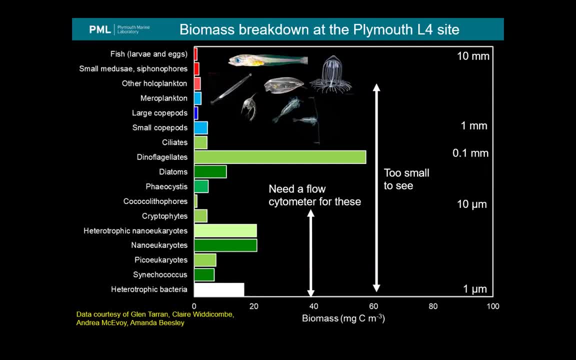 which are coded in green, The more Autotrophic tax, for example the diatoms and cyanobacteria, the synechococcus. dark greens, going to the more mixotrophic types, which are the paler colours. 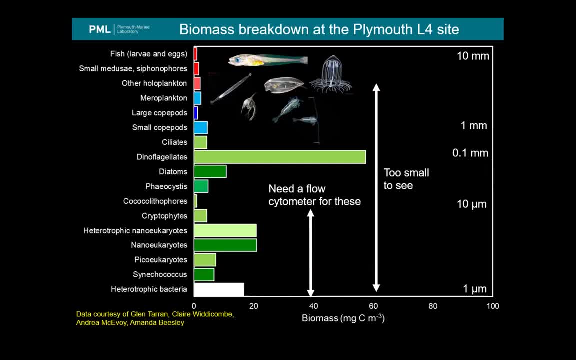 So I think the other thing to say about this slide is that the units of biomass are actually milligrams of carbon per meter cube, So they're tiny amounts per cubic meters of water. You're only getting a couple of milligrams Obesity Plankton feeding the rest of the food chain. 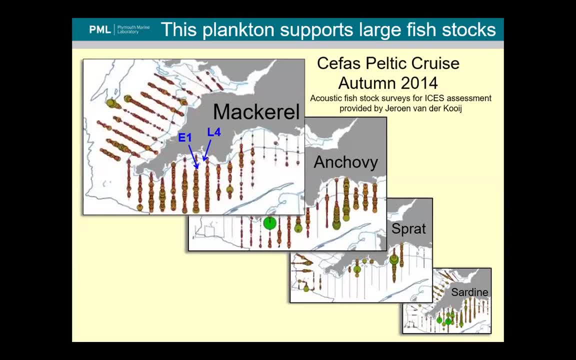 So that seems to be a little bit of a conundrum, because we know that there's quite big stock of fish in the West country. These are the CFAS cruisers. They repeat them every autumn And this is acoustic and net survey biomass of some of the fish in the pelagic. and these numbers, you know I haven't put a scale on them, but the actual 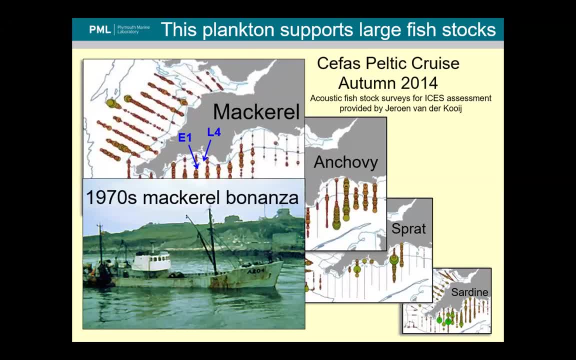 I think these are the actual numbers are around 430.. five years From that So, But this picture is a picture of the greatest amounts. The large magnitude of stocks of fish in the West country was brought home to me because I grew up in. 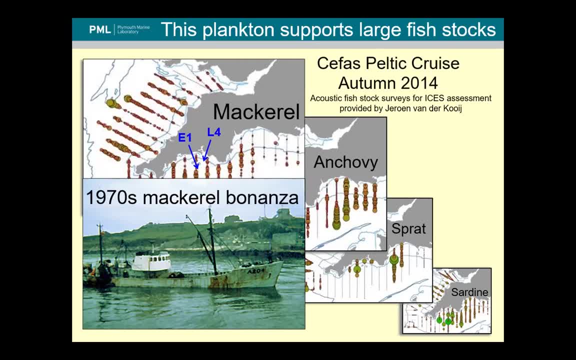 In the West Country in the 1970s And this is a picture of my father's trawler coming home, Hoyden into Mill Bay docks landing 140 tons of macro that they just caught in one night. And it's only by going out on this trawler that I could actually see with my own eyes what to produce those did you, soyGU? 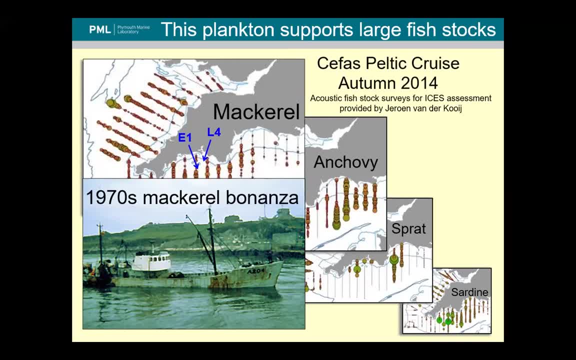 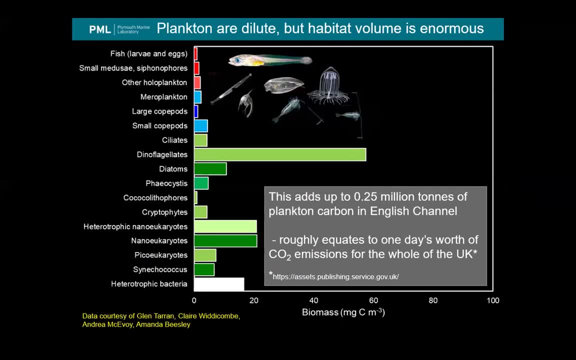 An Iowa sampling And there's actually a lot of butterflies, And yet they didn't actually have microplastics. There's a difference here. Another Point I'II throw today: Actually it wasn't destruction, food web, it was. So we've got a bit of a sort of conundrum because we've got tiny amounts of 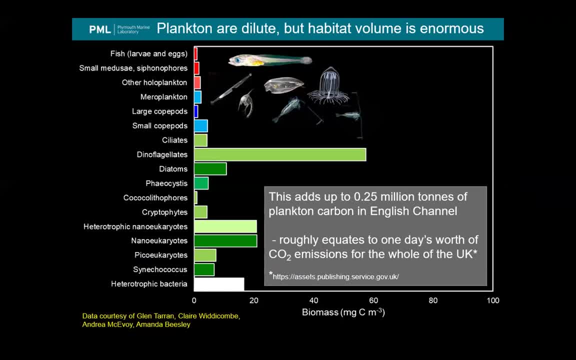 carbon in the biomass, of the concentration of the plankton is very, very small. but the answer is: the habitat volume is enormous. if you add it up- I've just scaled up with this calculation- 75,000 kilometers squared of the English Channel and the habitat extends down to. 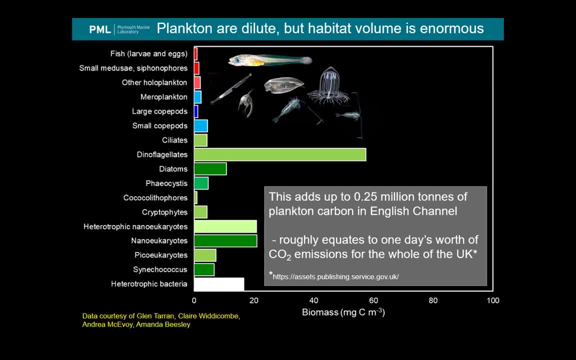 several tens of meters for the plankton in the productive zone. So if you add all that up, at any one time there was a quarter of a million tons of plankton carbon in the English Channel and to put a sort of human sort of scale on that it's roughly equivalent to the 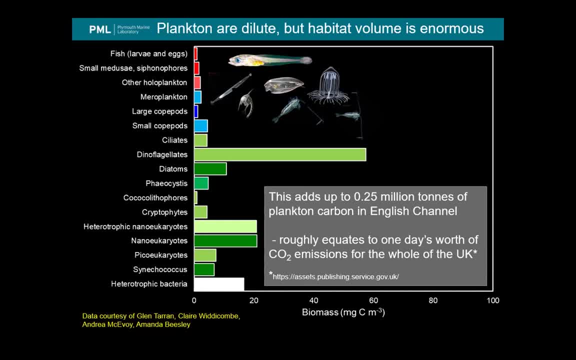 sludge. So you've got to remember that the the turnover of this plankton is roughly a day, roughly something like a day. so it's putting a sort of human value on it and there's a lot of interest at the moment in sort of describing ecosystem services and blue carbon and natural capital and a lot of emphasis. 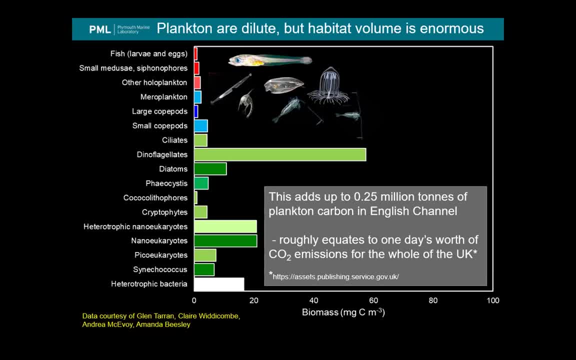 on them is on things like mangroves and seagrass beds And kelp beds. But the point is about the plankton. it's very dilute but the habitat volume really adds up, So it's a very large flux of carbon that we're talking about. 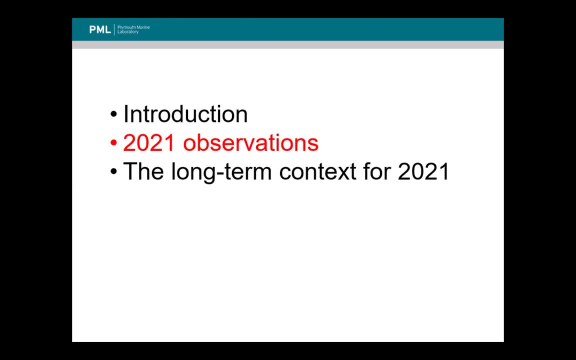 So that's a bit of a background to say why the plankton are worth studying in relation to climate change. How are these fluxes changing? So I'm now going to go straight in with the observations in 2020, 2021. 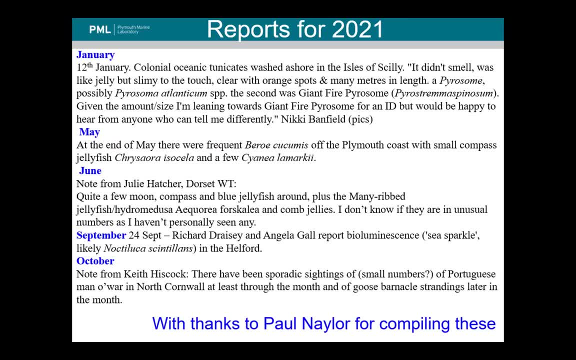 And these were compiled thanks to Paul Naylor for compiling observations that were sent in for the Southwest marine ecosystems. I'm not going to read these off. I've just selected here a couple of them running through the year, but I think the thing to note is that there wasn't actually a remarkable 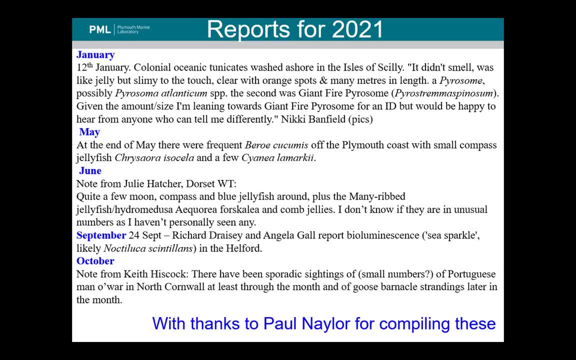 incidence of any of the particular plankton species, which was not a remarkable incidence of any of the particular plankton species we're talking about, which was not a remarkable incidence of any of the particular plankton species we're talking about often getting these reports of Noctiluca Sea Sparkle or some of the Gelatinous Sea Plankton. 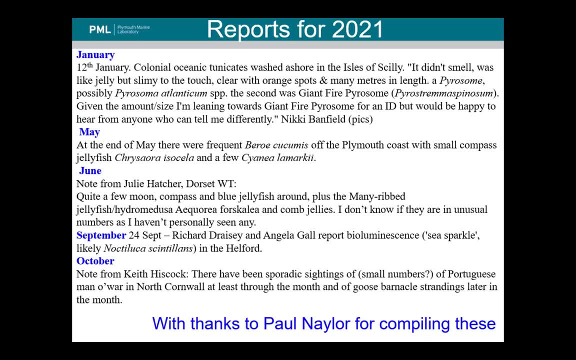 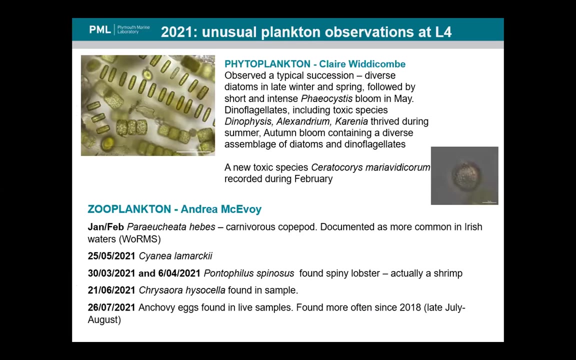 or some of the Portuguese Man of War, or By the Wind Sailors after the storms, so there's nothing really remarkable here. There was rather more compass jellyfish than is normal, but it wasn't a remarkable year, Likewise for the L4 Plankton Claire Widdicombe has described. 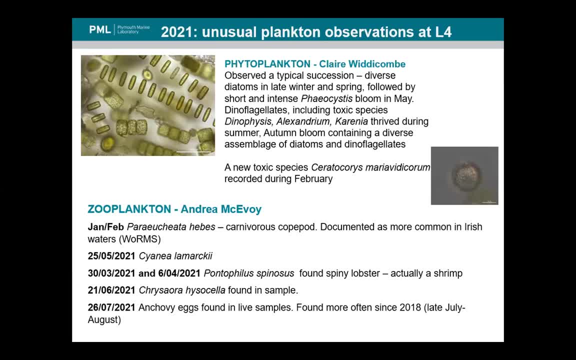 in the top paragraph here a fairly typical succession of Phaeocystis in the May and then giving way to blooms of Dinoflagellates in the summer and autumn. There was a new toxic species. this is a Dinoflagellate that she recorded in February. 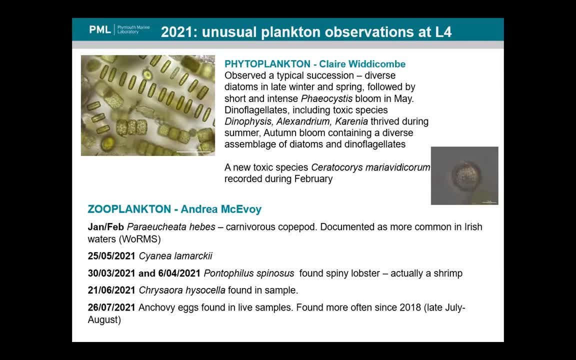 Likewise for the L4 Plankton, there was a fairly typical succession of Phaeocystis in the May and then giving way to blooms of Dinoflagellates in the summer and autumn. There was a few records but nothing really stand out. I should mention anchovy eggs found in the live samples. 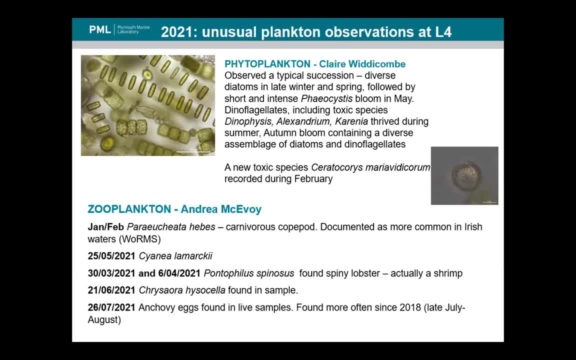 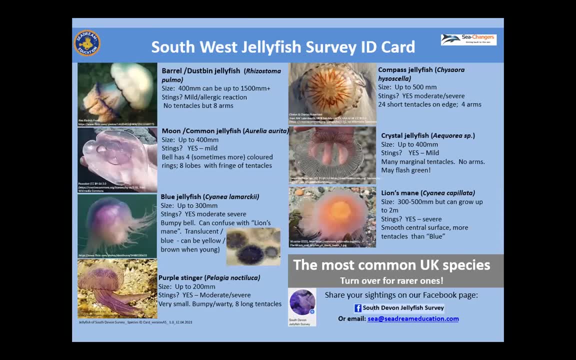 in the summer. That's continuation of a recent trend, possibly related to the warmer summer temperatures. So I'll stop there and just hand over. if, Jeanette, if you're around, do you want to talk about the South West Jellyfish Survey? We might need to open Jeanette's microphone. 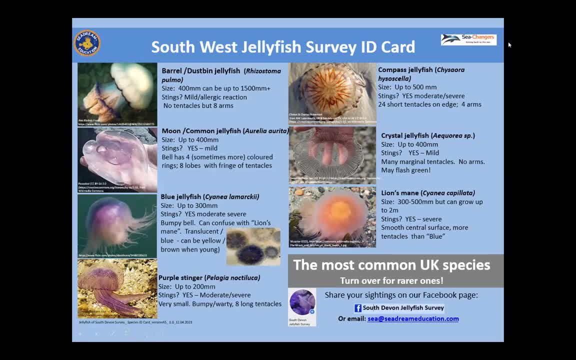 Jeanette, if you're there, could you unmute and I'll let you talk over these slides? You'll do a far better job of it than me, probably. I'm looking down the list for Jeanette Saunders. Yes, I've put a single image of the South West Jellyfish Survey. 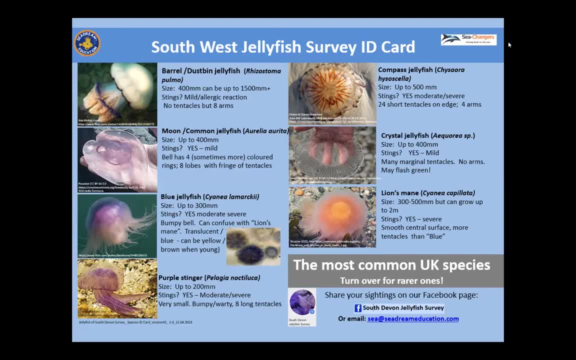 I think this one's a good one- allowed to talk, so, Jeanette, you should be able to use your microphone. can you hear me now? yes, indeed, excellent. thank you for unmuting me and thank you, Angus, for inviting me to talk. so in 2018, we were doing a lot of outreach and people were asking us. 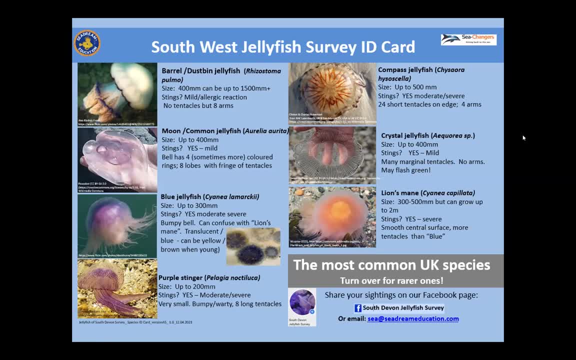 about unusual jellyfish that they were seeing. and these people were all people who were had a close association with the coast, so they were no strangers to jellyfish and we didn't have any answers for them. so we went out and did some surveys and we also launched a jellyfish survey. 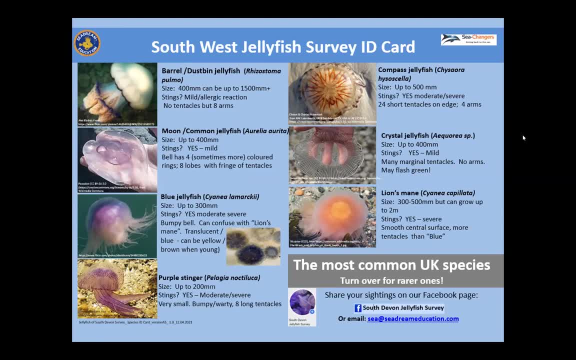 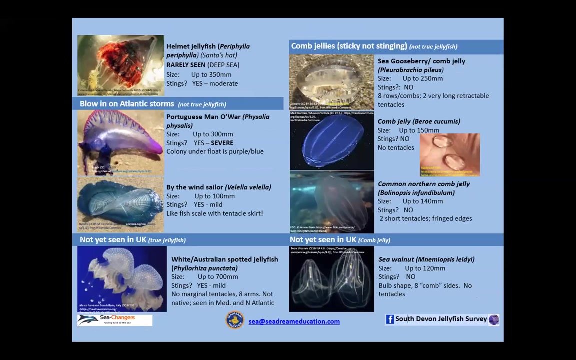 and we created some id cards with what we thought were the most likely species they would see, and so this is this slide shows, the ones that we thought at the time were going to be most common, um, and if we just go to the next slide, the, then it will show you the other side, um. so, Angus, could you just thank you um. so this, these are the. 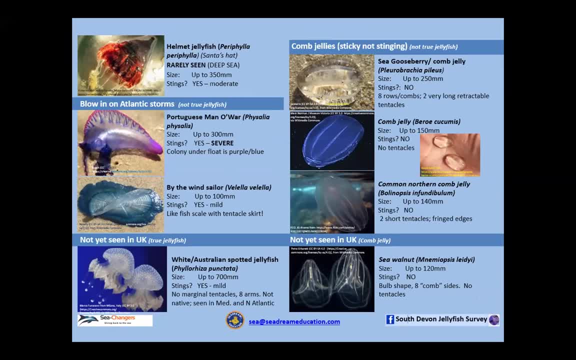 other ones that are less commonly seen, and you'll probably notice that they're not all jellyfish um. one of the problems we had was that we didn't really know what unusual things people had seen, so we didn't want to just restrict it to true jellyfish um, and this is the sheet we came up with. 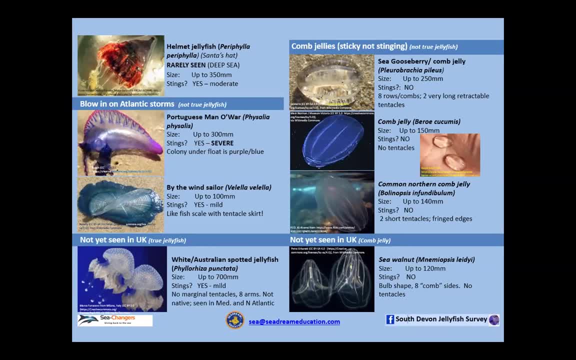 it's not perfect. um, there are some really good ones out there, but they either have a broader geographic distribution or they stuck to the true jellyfish. um, so we use these and our own surveys to collect data. so, if Angus wants to go to the next slide, 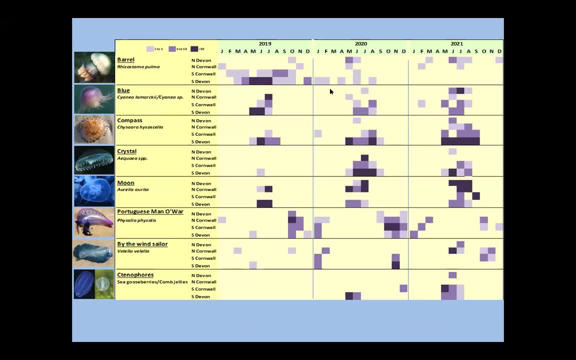 we'll go straight to the data um which I've tried to summarize here as best I can. so, across the top, you've got the years of data that we've collected, from January 2019 up to December 2021, and down the side you've got the species. 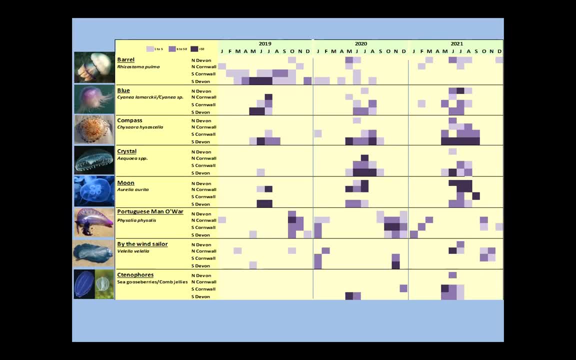 and we've also tried to sort of split it broadly into areas of the coast. so North Devon 끝, North Cornwall, South Devon, ander, South Cornwall, and then you've got little colored squares. um, so the colors reflect the maximum number of individuals that were reported by any one sighting in that month. 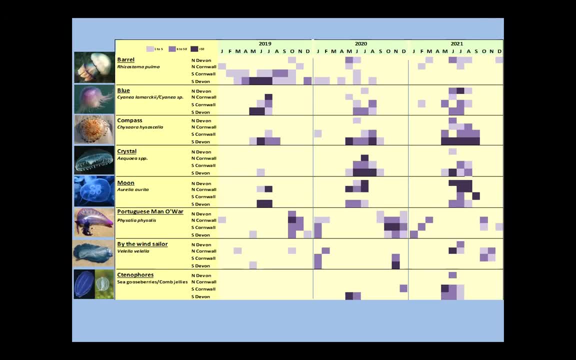 so they don't. we didn't add up all of the sightings, we just said, well, what was the highest number in any one event in the past? we just快esto put lots of numbers, medo. we just said, well, what was the highest number in any one event in that month? we just see it, i think two or three different kinds. 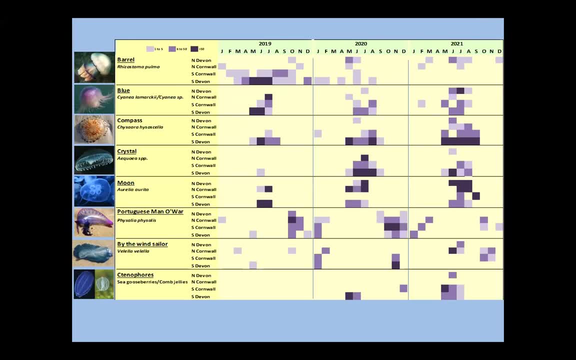 in that month. um, so the light gray would have been up to five sightings um, the purple would be anywhere between six and fifty, and the black is where more than 50 individuals were reported. if we go down them, the barrel jellyfish were quite interesting because anyone who was around 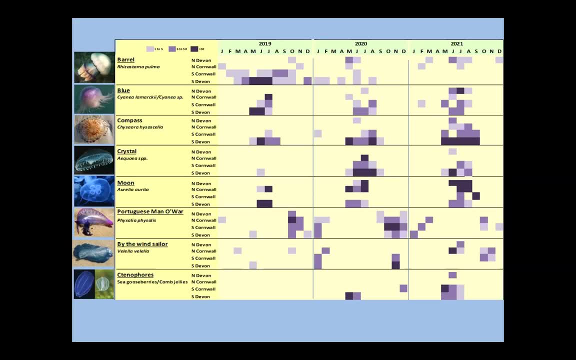 the coast in 2019 would have seen the barrel jellyfish. they were everywhere. they were washing up everywhere, um, but we haven't really seen that since in the same numbers. we have had anecdotal reports from local fishermen saying that they're still offshore in large numbers, and one person who 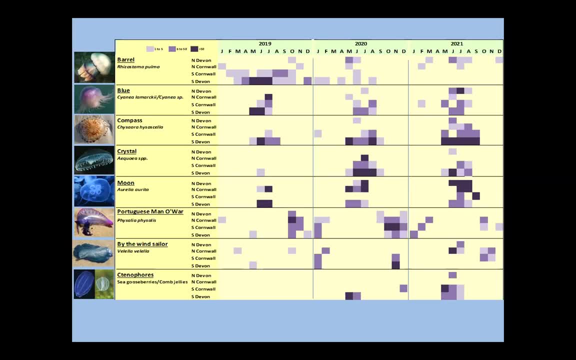 trolls falmouth bay- so he's been trawling there for 40 years- said that in the last 10 years out of those 10 years he has trawled up these mature barrel jellyfish by the ton in november for four years. so that that was quite interesting. but it doesn't really tell us much else about where they go. 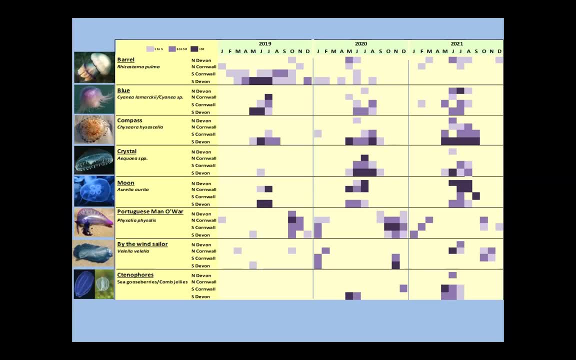 the blue, the compass and the moon jellyfish have pretty much the same patterns across all the coasts. um, there's a little bit of variation. the thing to say about the blue is that, although i've called it blue, we really don't know whether they're blue or lion's mane. 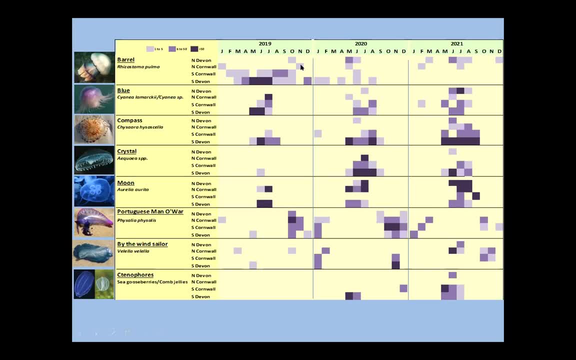 jellyfish because the juveniles are almost impossible for us to distinguish. however, we haven't had any verified reportings of adult lion's mane jellyfish around our coast in our data set, but we have had adult blues so it's most likely they're blues, but we can't be definite about that. um the crystal. 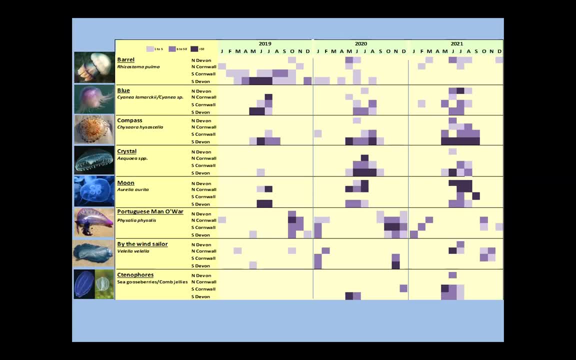 jellyfish is really interesting. it's not a true jellyfish, it's a hydrozoan um. it's really elegant and if you're lucky enough to see them in the water, they sometimes flash fluorescent green, which is where the original um green fluorescent protein that's used in microscopy came from. um, if you look in uk data sets for the 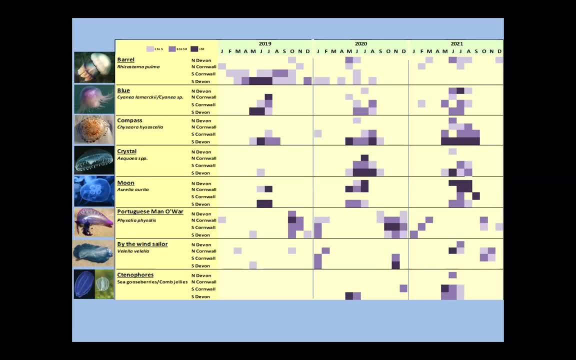 last 20 years they're very rarely reported, but if you go back to the 1950s and russell, you'll find that they were regarded as being fairly widespread. it's almost certainly at least two species, possibly more, that we're reporting um, and we didn't have many in 2019, but we certainly had a lot this year. 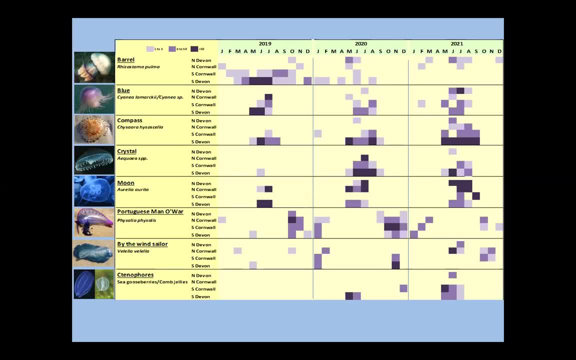 and in 2021.. sorry, 20, 2020.. um, the portuguese man of war and the by the wind sailor are also not um true jellyfish, and if you were to superimpose large storms on here, you'd see that they pretty much fit. 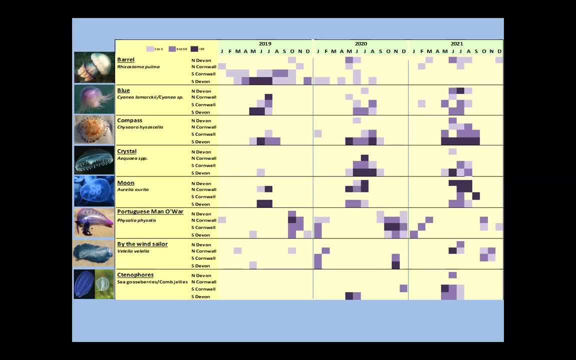 the pattern of washing up on the shores after the large storms um and in 2022. they've already been reported on every coast in the southwest region and, following the recent easterly winds, they've also been reported in areas like tour bay, where they don't normally. 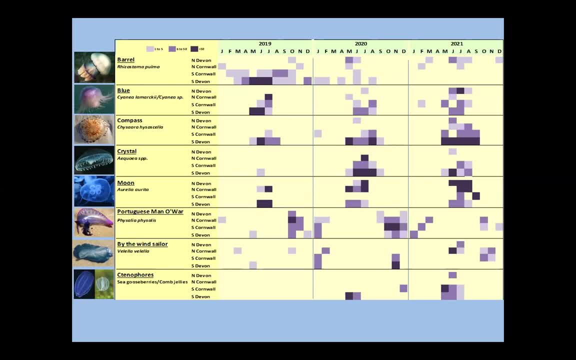 wash up. um, i personally think this- the tina fours- are really interesting. these are the seekers. frizz and cone jellies. um, we had almost no reportings until 2020, but in 2021 they have been reported pretty much everywhere apart from north cornwall. so prior to that, the reportings we had were really. 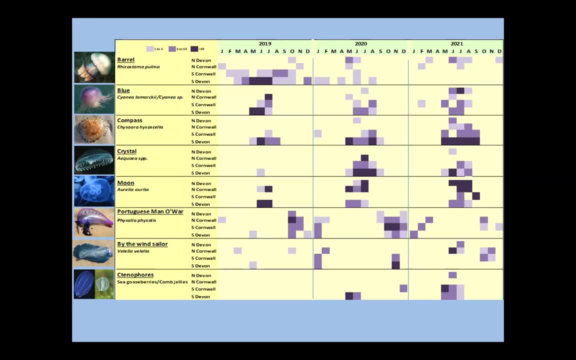 individual mass strandings, but in 2021. people have been reporting them um just looking in the water from harbour walls, swimming, diving, and there have been lots of them in the water actively, amongst other groups. jellyfish, um, the one that's missing from here. that is on our id card as a 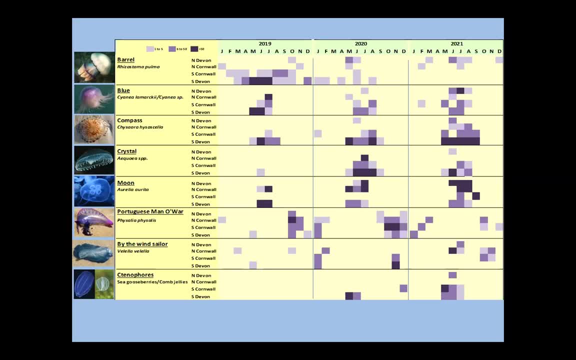 commonly expected species is the purple or mauve stinger, pelagia nottiluca um. although we've already a very significant list of species of jellyfish in eitherrakano and rhaea, there's also a lot of different species. there's a commonity of the hybrid species of jellyfish that we've mentioned. in a previous report i think there is, for example, the oval blue stinger. so those are the more independent und structures that come from portal dernier and some of these species are more know as of late of theexisting species. you might hear of jerry dry um the blue tilaka, like word that comes out of jerry промars. 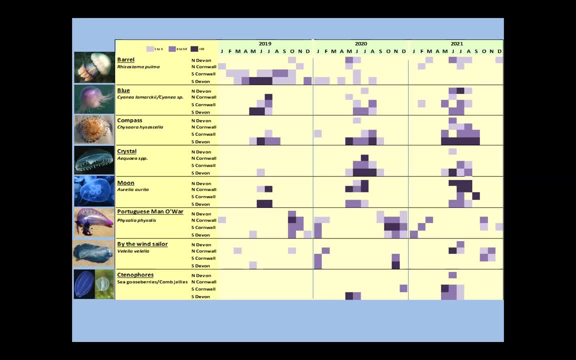 And although we had a few reports of this, when we looked into them they were definitely misidentifications and they were actually blue jellyfish. But there are reliable historic records of large mass strandings of this species, particularly in South Cornwall, So we don't know where they are or what's happened to them. 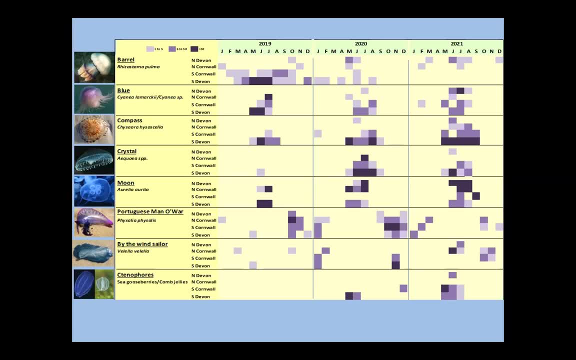 So, although we launched this as a citizen science survey, a lot of the data that I've presented here was collected by actively stalking people on Facebook and searching for jellyfish sightings and seeing what's been entered, And so there are lots of problems with this sort of data. It gives a really nice overview of where things have been seen and sort of a feeling for where they are, but it's not very precise. 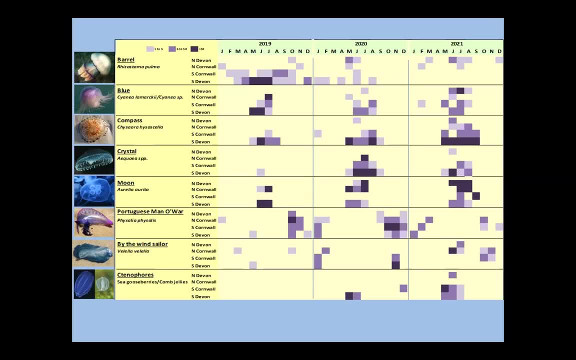 If we use the social media, then we have to try to verify it. So we only include reports where we have a photograph, a date and, ideally, a little bit more information. but we definitely need a place, a date and a photograph. 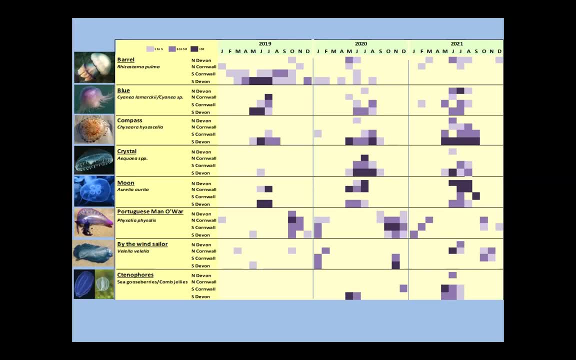 We do also include ones that are reported by people that are known to be fairly expert, but that's unusual, And so And so, And so, And this data set relies heavily on strandings And, as a result, there's lots we don't know. We don't know how many jellyfish are actually out there. We don't know whether the numbers are changing. We don't know whether climate change will favour jellyfish or a particular species of jellyfish- We haven't seen any invasive ones yet, but they could arrive. And we also don't know whether the ones we see are fulfilling their whole life cycle here, because we don't know where the juvenile polyps are. 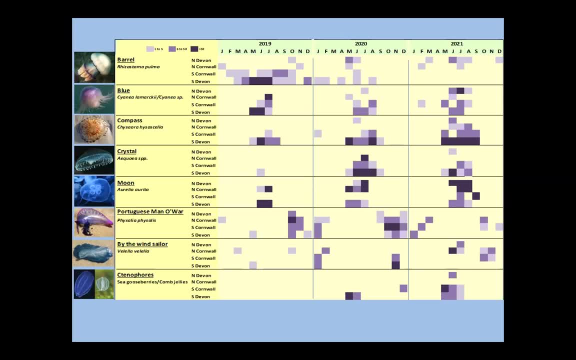 So we are going to keep the citizen science going for as long as we can, and we also have supplemented that with some work on environmental DNA, so testing the water for jellyfish. So I just want to say a big thanks to the MBA, who provided a small fellowship to Michelle Kiernan to do some of that work, and the staff at the MBA, PML, Amanda Helen Rowena and the staff at University of Plymouth who've been fantastic. 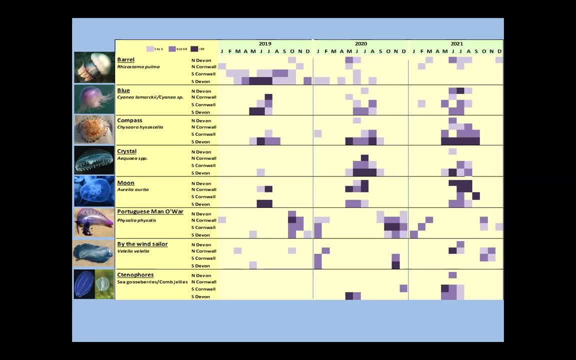 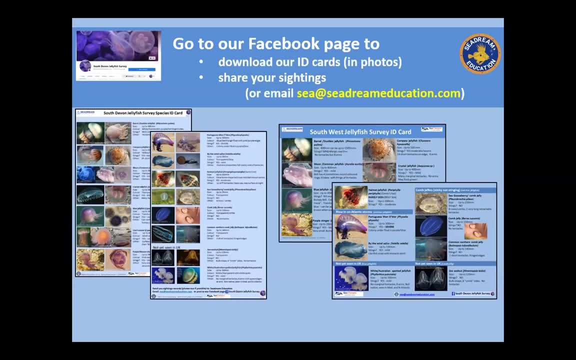 in supporting Michelle in that work. And if we quickly go to the last slide, These are just our ID cards. There are some large ones which we found people felt were too big for them to carry around, so we've got the small ones. 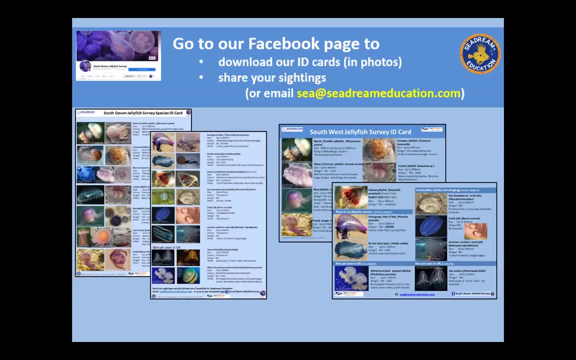 They're all on our photos on our Facebook page to download, and we have a small amount of funding from Sea Changers- a great little charity- to print these and provide them free of charge to people And we are planning to share them. We're going to share this data with other people, So we have been in touch with Marine Conservation Society, but that was pre-COVID. 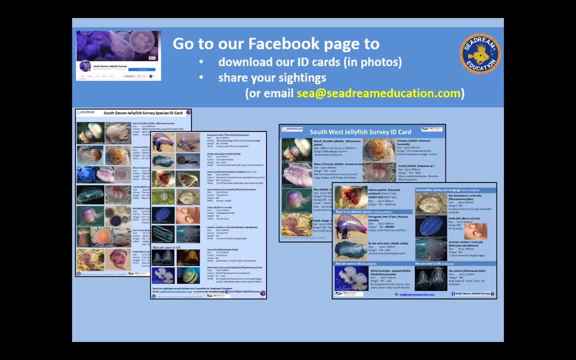 And we do have to really clean up our data set and make sure it's in a really good condition so that we can share it with them with confidence in the data quality. And thank you to Angus for letting me talk about our study. Please give us your sightings So I'll hand back to you, Angus. 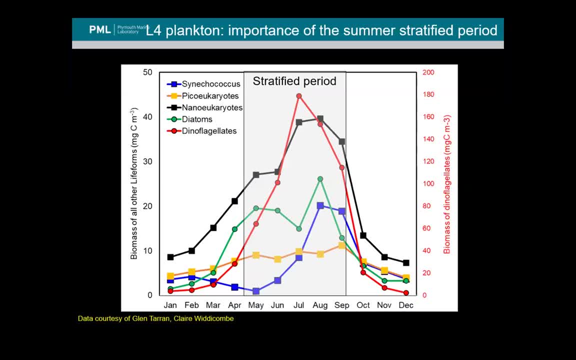 Well, thank you very much, Jeanette. It's a really good compliment to have this Southwest jellyfish survey alongside things like the point sampling at the L4 and E1 sites that I'm describing, because the time series is a nice long time series but it's not including these large jellyfish and it's only in one place, So I think they fit together really, really well. So I'll just carry on a bit more about the long time series at the L4 site. 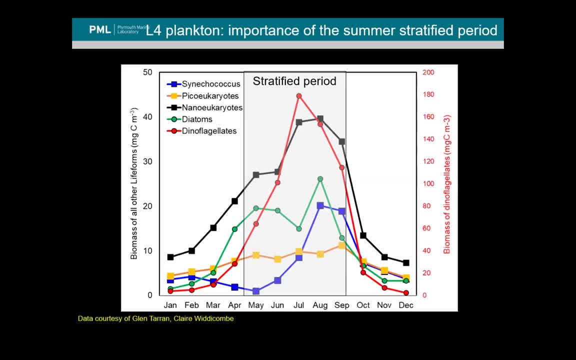 But before doing that I just want to describe the seasonality of the site. As Tim said, we've got this summer period, typically May to September, where the system gets stratified. there's a thermocline and that runs the system out of nutrients and the small supply of nutrients in this warm summer stratified period goes straight into the plankton. So I'm going to describe two halves of the year, the stratified period and the rest, in the following slides. 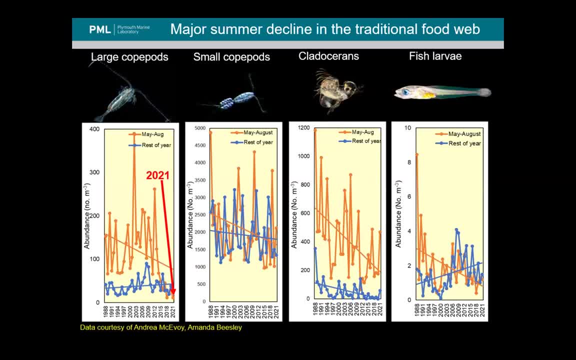 So this is the 30 plus year trend of some of the links I've just described in that classical food web. This is provisional data from 2021, but for the large copepods, which is strongly dominated by the Calanus helgolandicus, that's the left hand plot. 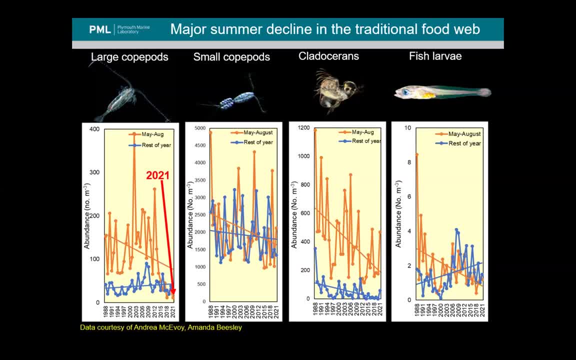 This is data from Andrea McEvoy and Amanda Beasley And that shows a real step change in this summer stratified period. that's the orange line. the abundance has plummeted since about 2012.. And that contrasts with the abundance in the rest of the year, which has stayed relatively constant. and that pattern of 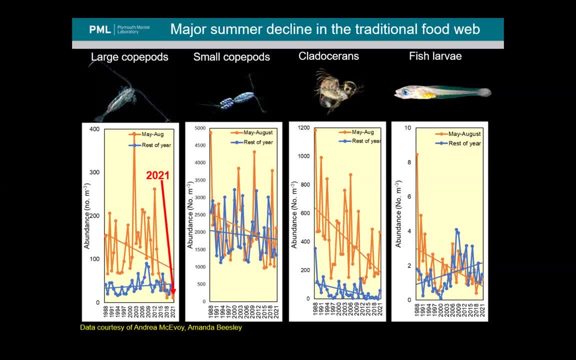 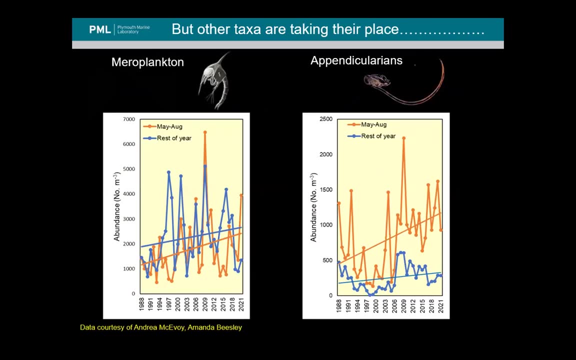 a steep decline in the summer compared to the rest of the year is mirrored by other taxa, for example, the small copepods, the cladocerans and the fish larvae. A completely different trend is seen by some of the other groups, and this is the. 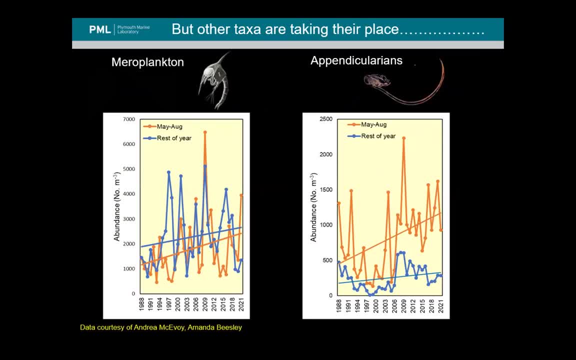 meroplankton, that's the pelagic larvae of benthic invertebrates, and another group, the appendicularians. They've increased more in summer than in the rest of the year, so they're almost like replacing the links in the classical food web. So the thing that unites these two taxa. 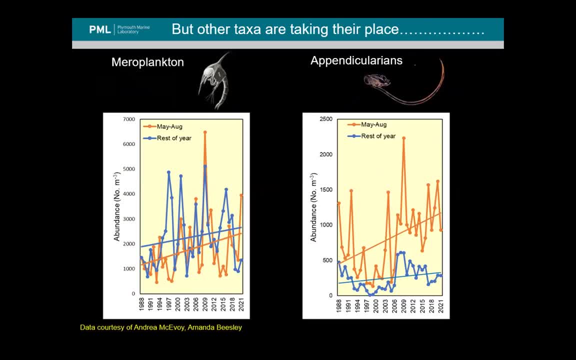 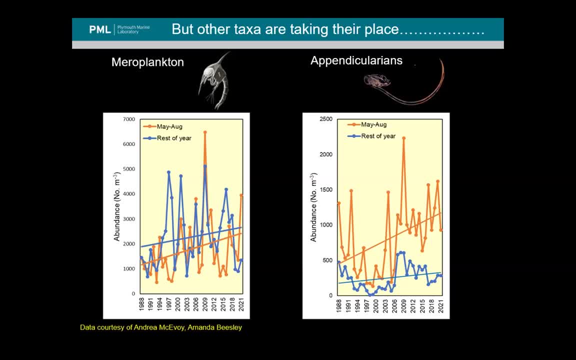 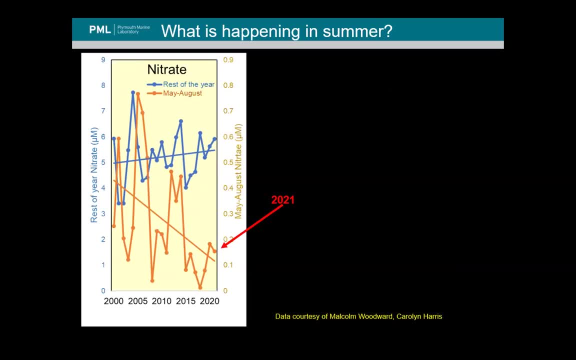 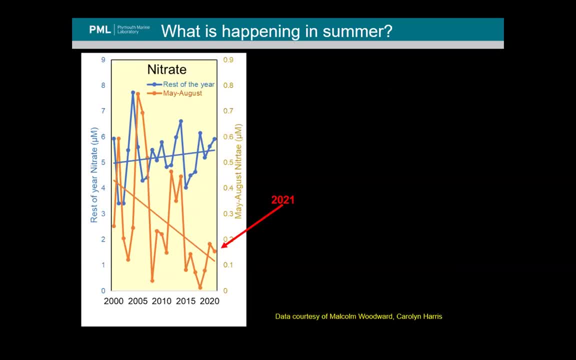 it again into the May to August versus the rest of the year. The rest of the year the nutrients have stayed fairly high, but in this nutrient limited summer warm stratified period the availability of the nutrients has dropped quite dramatically. So that is a suggested cause of some sort of disruption in the food chain. So we looked at the next level up. 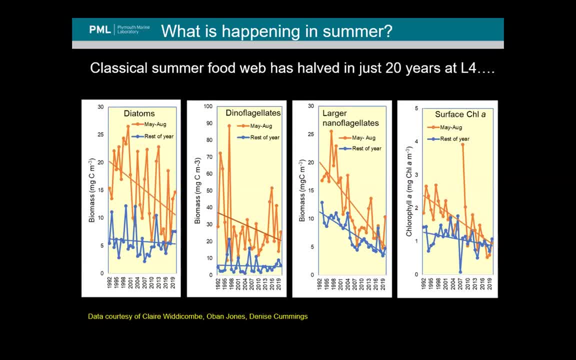 for these taxa, which rely on relatively high nutrient concentrations. They're inefficient at getting low nutrients compared to some of the smaller cells with a bigger surface area to volume ratio. So these are the larger phytoplankton that Claire Widdicombe counts with her Lugolz counts. 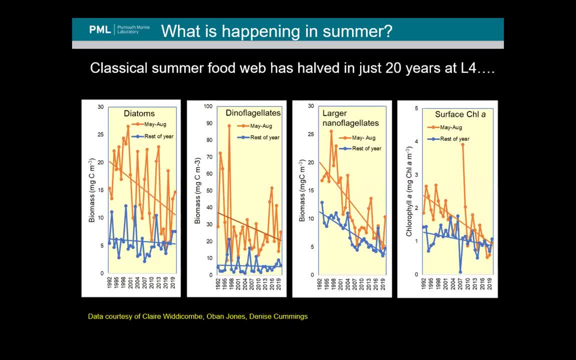 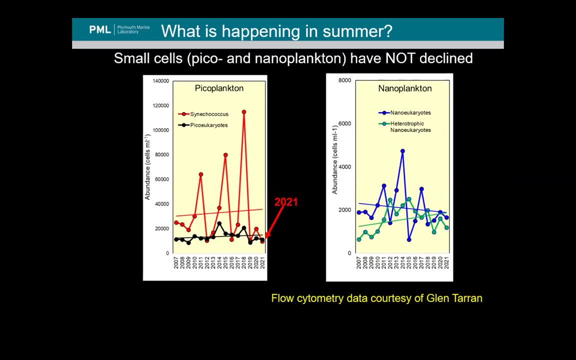 So the diatoms, the dinoflagellates and the larger nanoflagellates that Claire counts have all declined quite dramatically in this productive summer time of the year. These are the small cells that you need a flow phytometer to count. 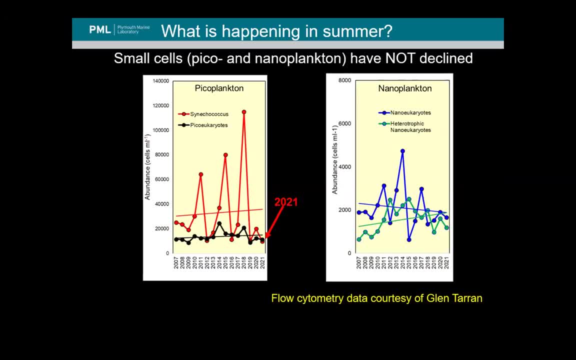 This is Glen Tarran's data on the pico and nanoplankton and that's running from 2007 to last year. These are surface values and these show that these smaller fraction haven't declined like the bigger diatoms and dinoflagellates, So we're seeing a major 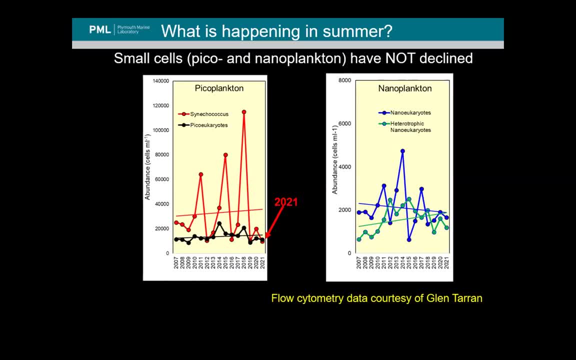 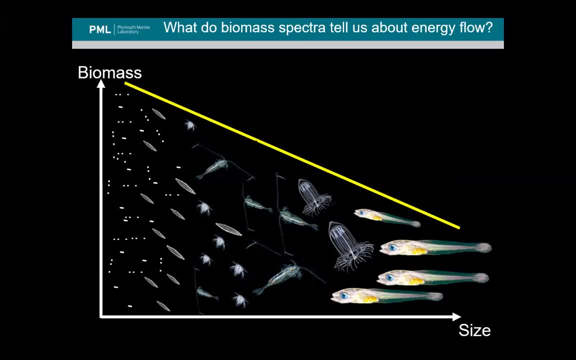 disruption in the food chain. that's related possibly to some of the size issues. We had a little bit more of a detailed look at this sort of body size approach to understanding what's happening at the L4 cell, And this is using size spectra, which is basically based on the principle that, as you go up through 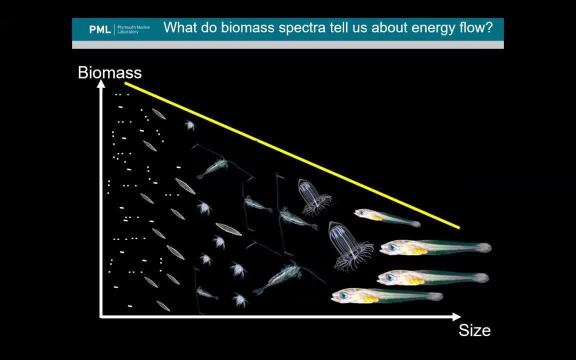 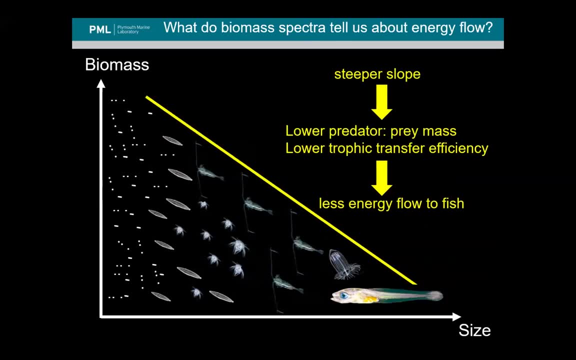 the food chain. the animals get larger but the total biomass of those animals gets progressively smaller, And the rate of this attenuation in biomass is a measure of the energy efficiency of the food web transfer. So a steeper slope means a lower predator prey mass ratio or a lower traffic. 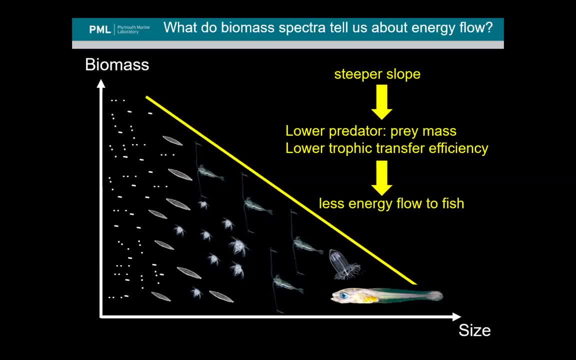 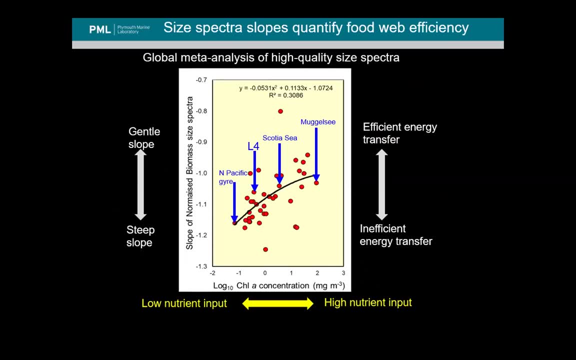 transfer efficiency, Either of which mean less energy is flowing up to fish. So we look at the L4 site in relation to a literature compilation of all available high quality size spectra. So on the y-axis is the slope of these size spectra and on the x-axis 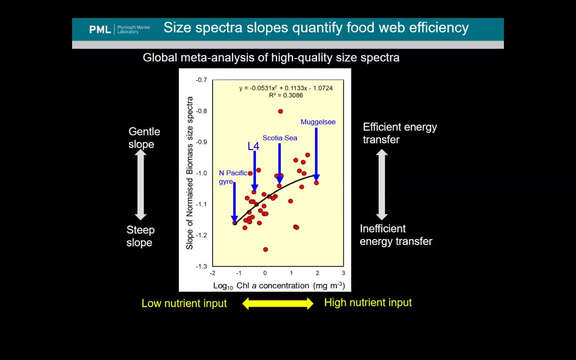 is the nutrient input and I've proxied that here by the annual average chlorophyll concentration. So this is called a meta-analysis. So this is work in progress, But basically points in the bottom left of the plot, for example the North Pacific gyre. 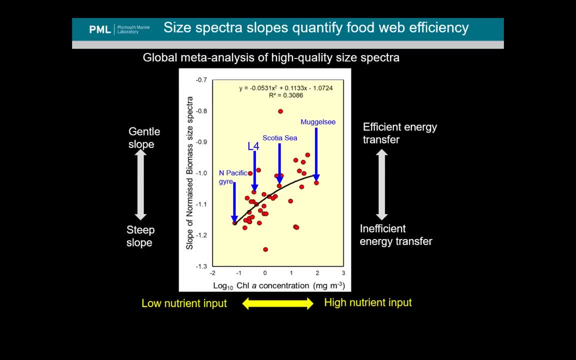 These are the so-called deserts of the ocean, which are receiving very little nutrient input. They've got a steep slope so it's inefficient energy flow through the planktonic food web. On the opposite extreme, the top right, this is a land locked well inshore lake. 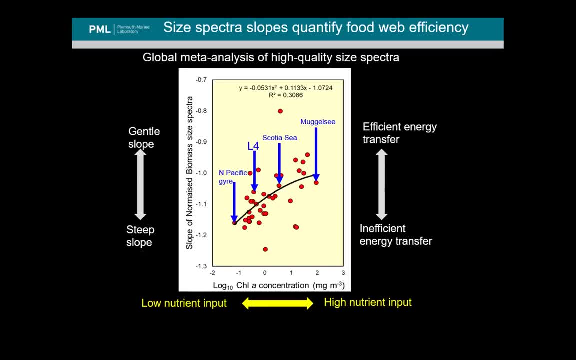 I'm sorry. It's a lake in north west, in northern germany, which is in agricultural land, rich nutrient inputs and very high chlorophyll and relatively efficient energy transfer through the food web. elf falls somewhere in this spectrum. so what you would expect with climate change, it's it's tending in temperate latitudes. 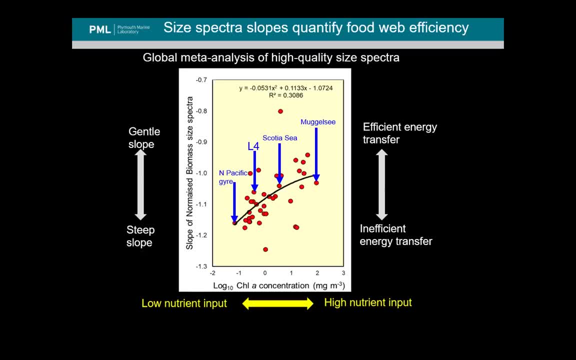 to increase the degree of stratification and that is concurrent with an increasing nutrient limitation in summer. so it's pushing them from the top right to the bottom left. so we can measure the inefficiency in the energy flow in relation to the climatic change. so a 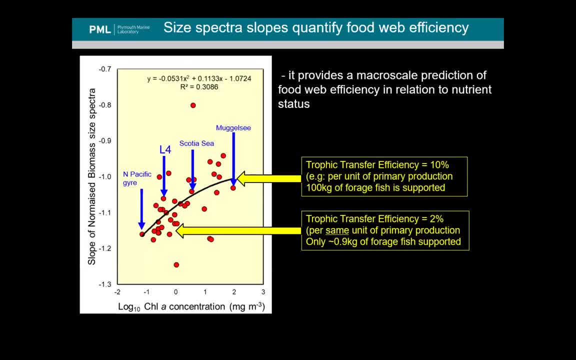 rough, rough sort of indication. top points in the top right are a relative to the efficient energy flow through the food web and the bottom left. not only is there less energy going into the food web, but the trophic transfer efficiency is also dropped. so it's a double issue as you reduce the nutrient input. so to sum up, at the elf. 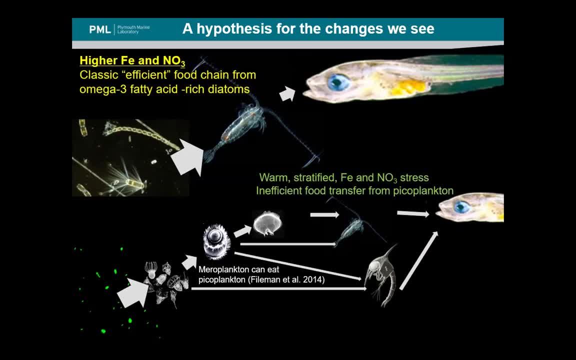 falls site. we seem to have moved away from this sort of simple textbook idea of a short, efficient classical food. chop practicing food. Hey, the end time, the 24 hours, which requires conversion times with contrasting features, chain to something that is dominant. well the um, the nutrients are more limited in the summer. 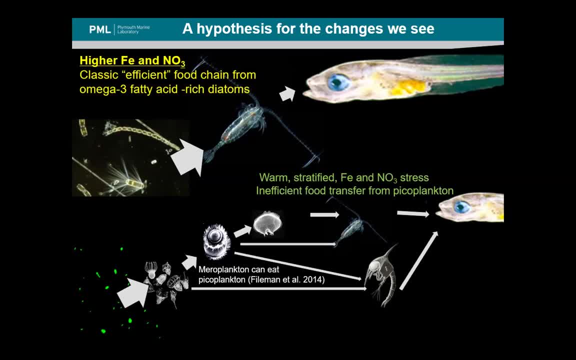 that's favoring the smaller cells and the grazers that are can be specialist on eating these smaller cells. so, for example, it's favoring summer increases in meroplankton and these appendicularians that can eat micron sized food particles. so it's a relatively inefficient energy flow that we're. 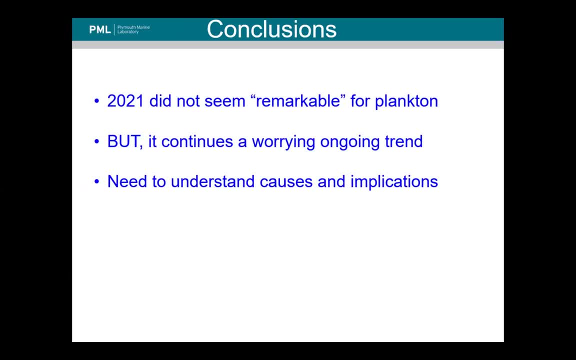 moving towards with the climatic warming. so, um, just to sum up, um, 2021 didn't seem to be particularly remarkable for plankton. um, we're going to compile all of the observations into the annual reports and the main thing from the time series is that the um it's sort of like the new normal it's. 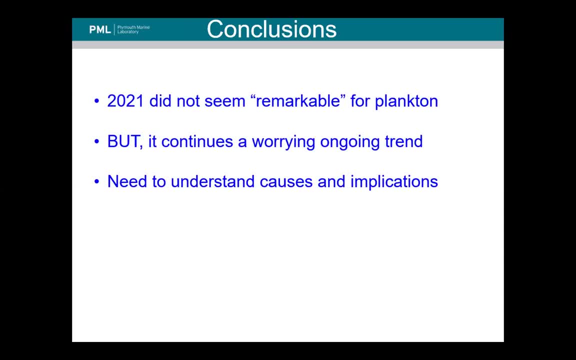 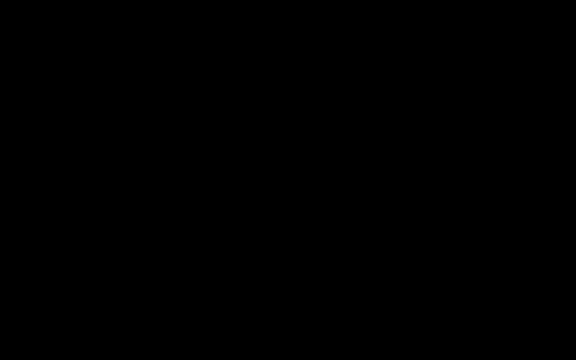 the continuing of a ongoing trend of smaller cell domination of the food chain, and it's still work in progress to try to understand both the causes of it and the implications of it. so that's it, thank you very much. i'll stop sharing and that's me done. thank you very much indeed, angus. um, i'm not actually seeing any questions. 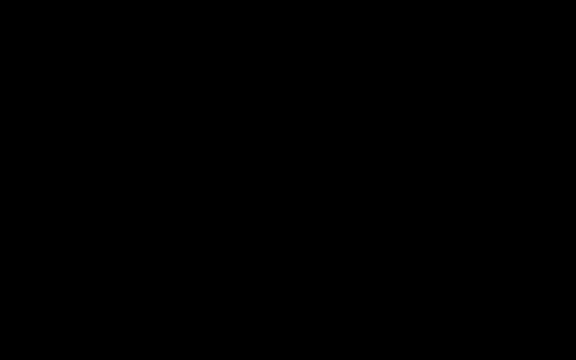 or additional chat. i've got one question pop up now, um about iron deficiency. are there measures of iron at l4? um, not that i'm aware of, um. i know that um the group um simon usher from the university of plymouth, um was interested in measuring iron at l4 and we certainly would. 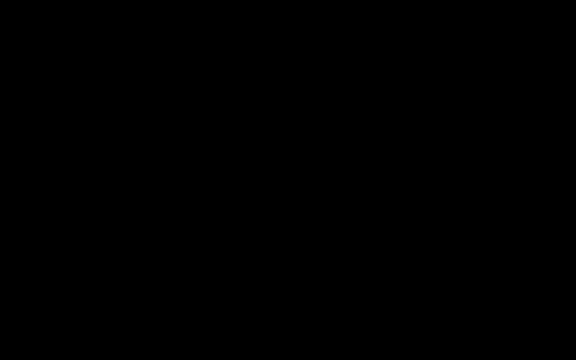 really like to, because, um, there's an indication that um, not so much at l4, but the offshore site e1, could become iron stressed in some years. um work in the shelf c biogeochemistry program has shown that even waters um in the celtic. 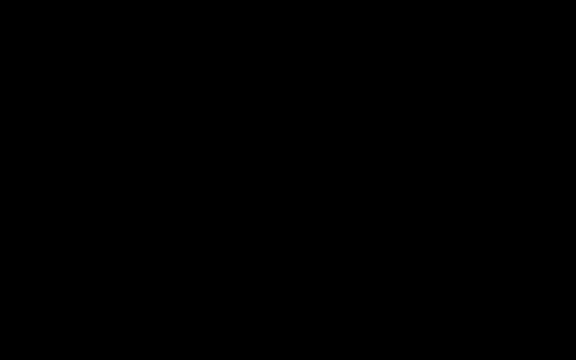 sea can become iron stressed. it was initially thought that iron stress was a sort of um something that was only happening in these remote ocean gyres, but i think people are finding it's becoming a lot closer to home, so it's likely to be a co-limitation of iron and a series of other nutrients. 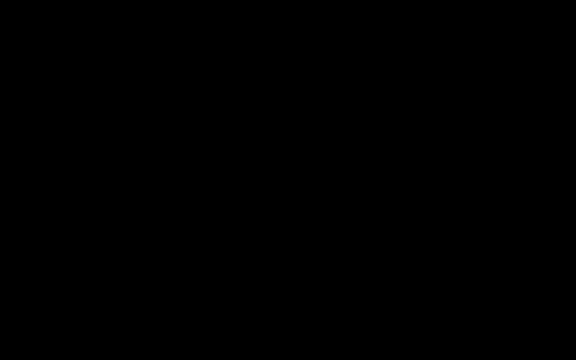 in the future. so that's a good question. um, i'm going to take the privilege of um being uh live to actually ask something about the larvae of spiny lobsters, paloneurus eliphaz, when people were working on the different stages of uh development in a larva which stays in the 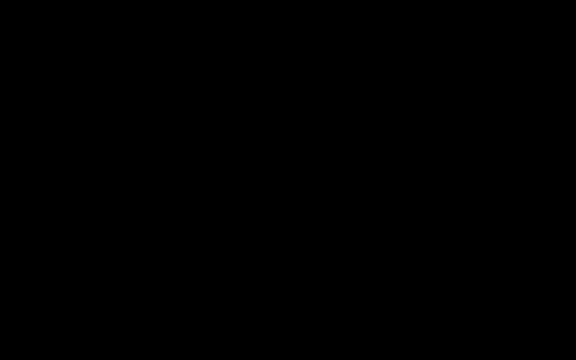 plankton for about 150 days. they seem to have no problem catching them at the eddystone or round about the eddystone. do you ever get a phylosoma larvae of paloneurus eliphaz in your plankton halls? um, i'll have to. um ask andrea um mcavoy, our chief zooplankton analyst, um in particular, i think um. 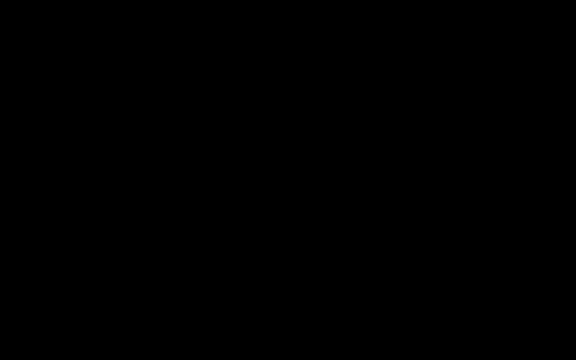 in her observations. um, there was um some reports of larvae, um, so we'll have to go back through them. andrea's just said: only very occasionally. um, all right, but they are. they are very occasionally found still, but um, who knows what effort the 1950s biologists put into catching 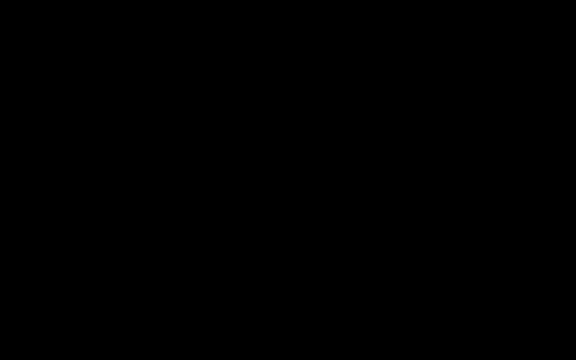 them, but certainly seems if they had no problem. so thank you very much indeed for that. i haven't got any more q a questions, so i'm going to uh, unless the presenters have got anything else that they want to, um bring to the audience, the participants attention. um, i'm going to switch back to um square. 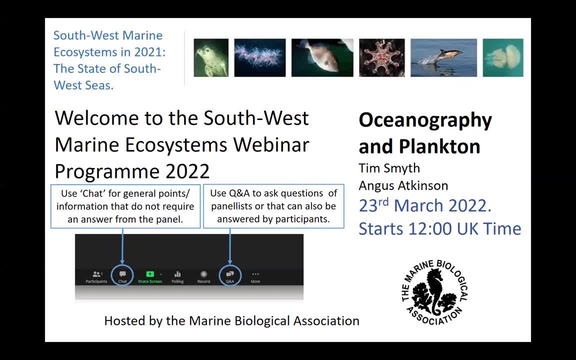 screen he says: hopefully, i've managed to do that, keith, you're just on the welcome slide, that we can. yeah, well, that's all right, i intend to be on the welcome slide, but it hasn't got a green border around it, which is supposed to have, which is. 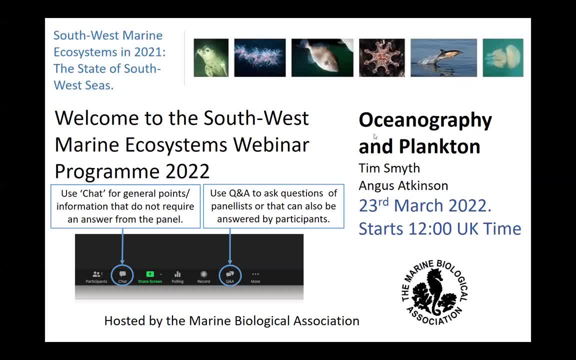 confusing me. so, um, thank you very much indeed to all of our speakers and for participants for joining in um what we're doing in southwest marina. you can see where we are- hello there- on the website. i want to let you know that i was fortunate to be.